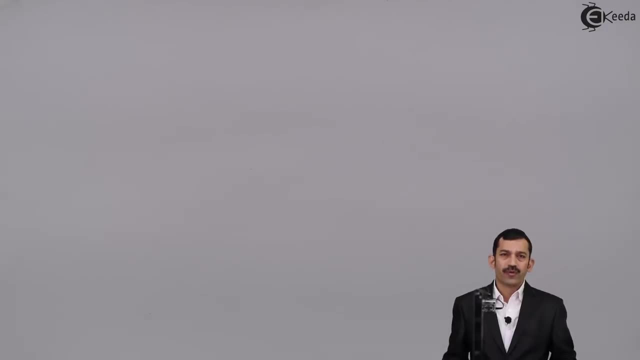 two bodies having some masses say M1 and M2 collides with each other, then exactly what happens If we will assume that this one is one body, say this one is a bat and say this one is other body, which one is nothing but say ball, Now, this one is body. 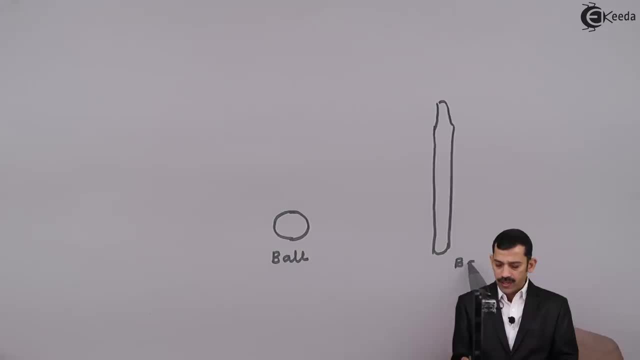 one say ball, this one is next. body say bat, say this one body is one, this body is two. This ball means body one having some mass M1, this bat having some mass M2, this bat having some mass M1, this bat having some mass M2,. 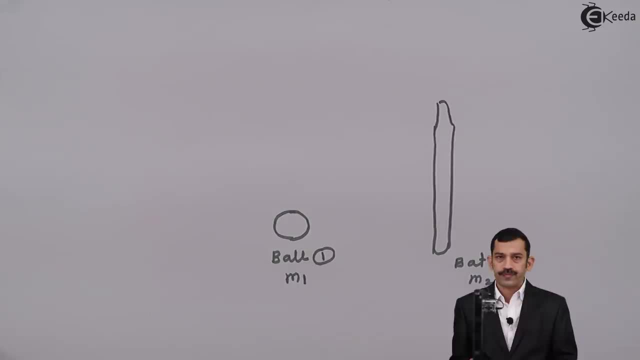 means body two having some mass, M2.. Now, if this ball moves in rightward direction and then this ball strikes the bat, Now, when this ball strikes with the bat, what forces are developed or what reactions are developed? that one we will see When this ball strikes. 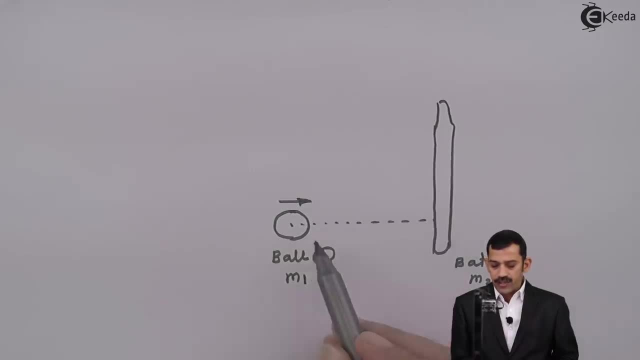 with the ball. what diagram I am drawing? This one is when this ball is in contact with the bat, When ball strikes, then ball rebounds. When ball rebounds, this bat or this batsman also experience some jerk which opposes or which acts in opposite direction. That means, when this ball strikes with the bat, some. 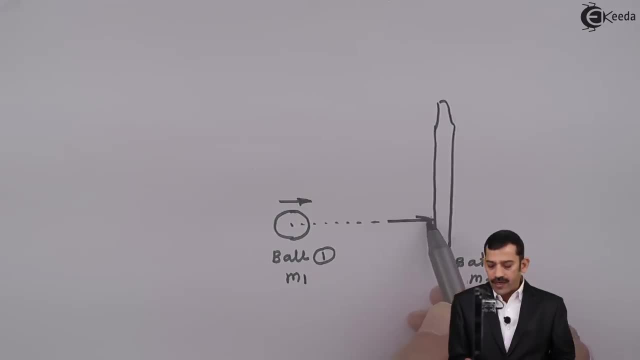 force is exerted by ball on the bat. This is a force exerted by ball on the bat, say in rightward direction. Similar force, same amount of force, same amount of reaction is developed or acts by the bat on the ball. That means force exerted by bat on the ball. 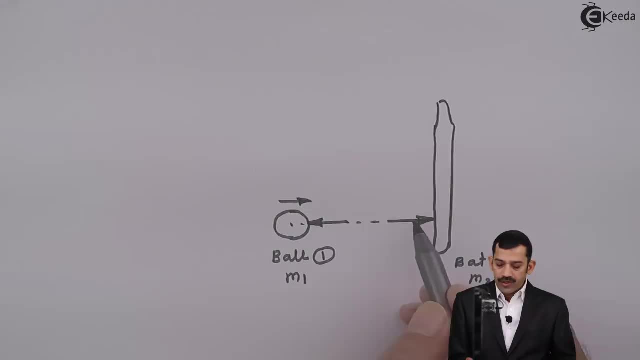 is in leftward direction, As this force, which acts on the bat, is exerted by ball, means body one on body two, that means bat. Similarly, what force we are getting here, we are getting here is F21, meaning is what Force exerted by body two on body one, that means force. 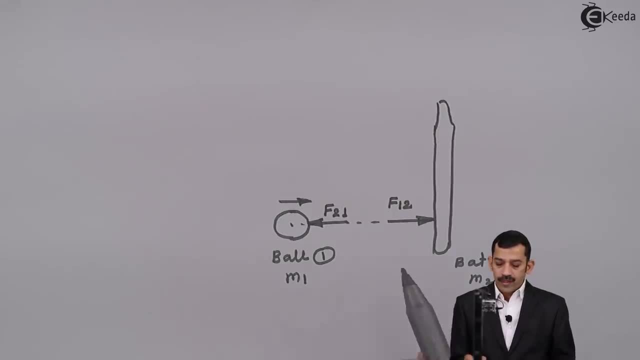 exerted by bat on the ball. Now, as this forces are exerted, this forces are exerted in what time? When ball strikes with the bat, then ball remains in contact with the bat in short interval of time. Therefore, such force which is developed, which is a large amount of force, 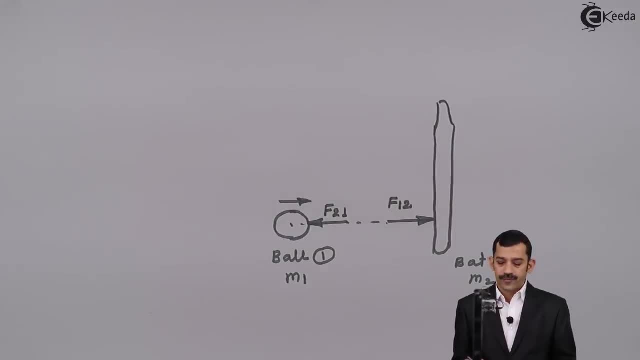 which is developed in a short time interval, then such a force is called as impulsive force. That means F12 is impulsive force as well as F21 is also impulsive force. That means what is the meaning of impulsive force? The large force which is exerted in a short interval of time, when two body collides with. 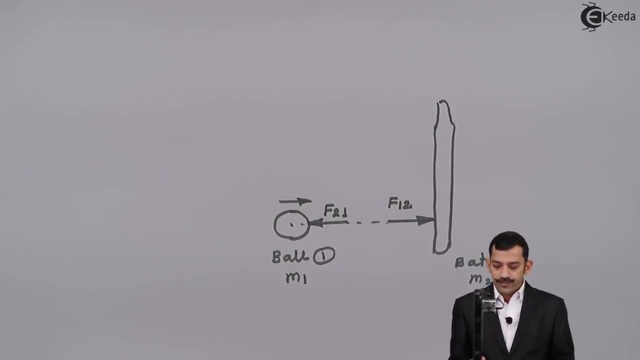 each other. Therefore, first term is impulsive force. Next one: this force acts on these bodies in a short interval of time, product of this impulsive force, and the time interval in which this force acts is called as impulse of force. That means second term is impulse of force. 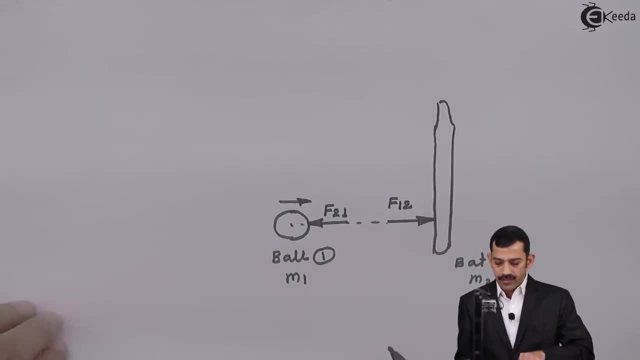 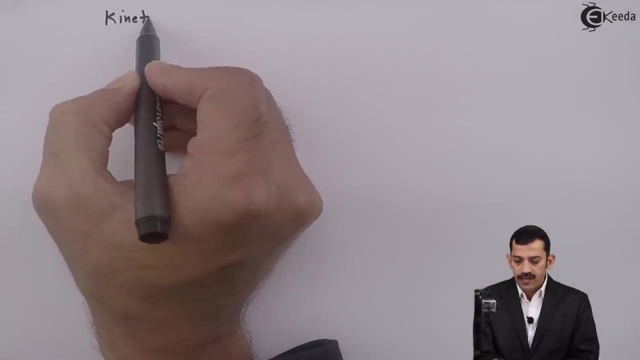 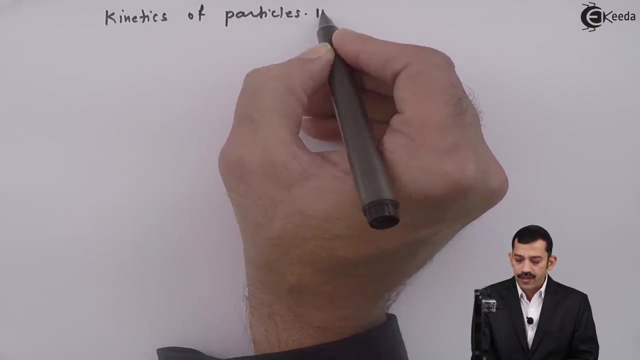 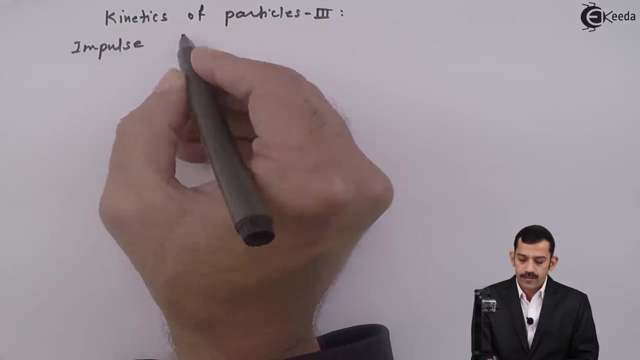 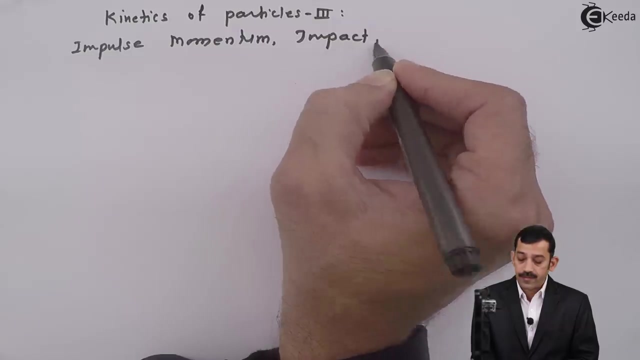 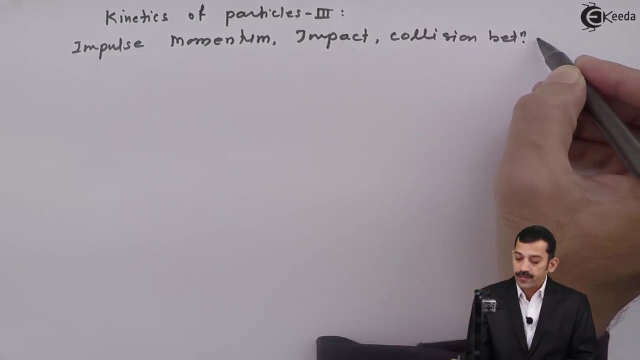 Let's write these terms one by one: See here on next page. So this is impulse of force, Kinetics of particles. three impulse: momentum, impact. it is nothing but collision, collision between Elastic bodies, First term. what we will discuss is impulsive force. 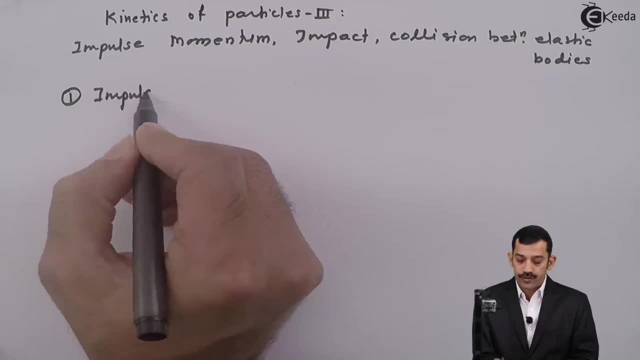 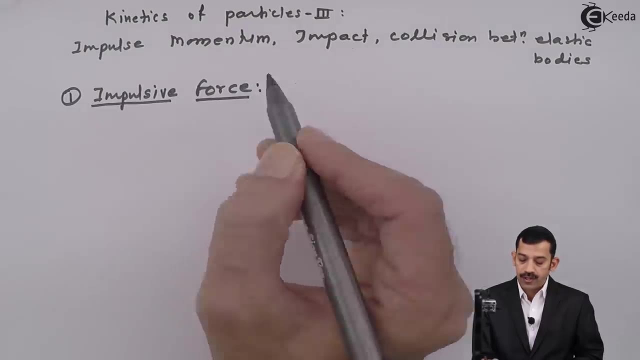 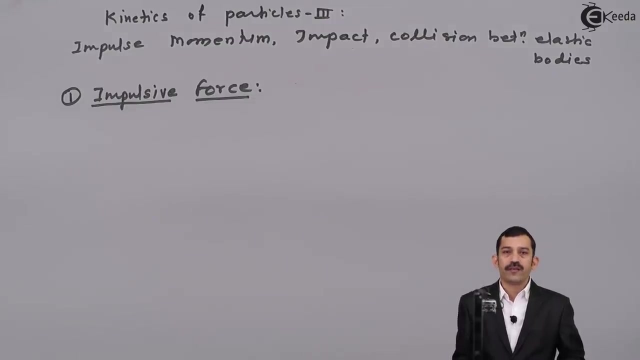 See number one, impulsive force. Now, this force, impulsive force, means which type of force? Impulsive force is a force which is developed or exerted. So impulsive force has two bodies, collides with each other in a short interval of time. 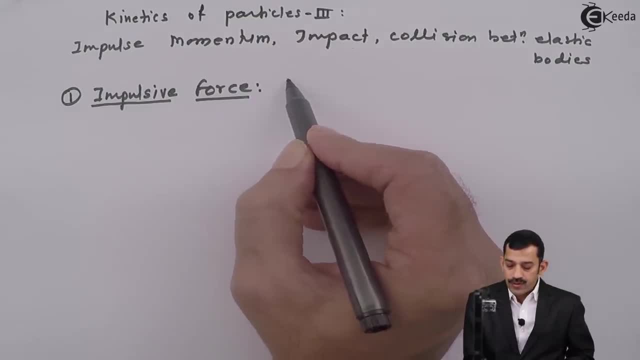 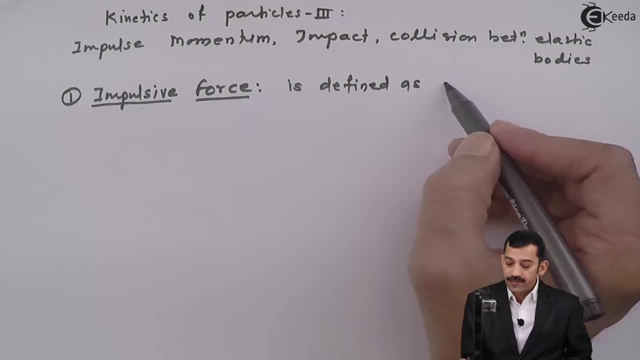 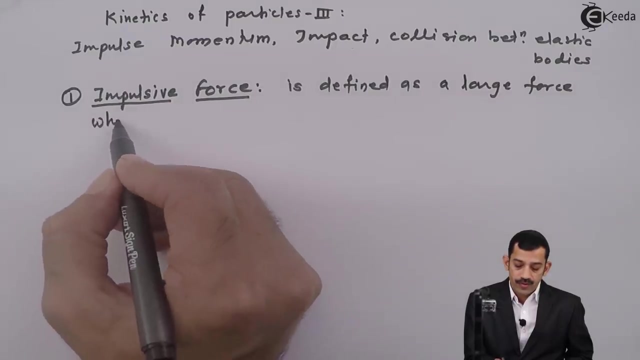 That means impulsive force, if you want to write. Impulsive force is defined as what Impulsive force is defined as. Impulsive force is defined as large force. Large force which is exerted. So large force which is exerted. 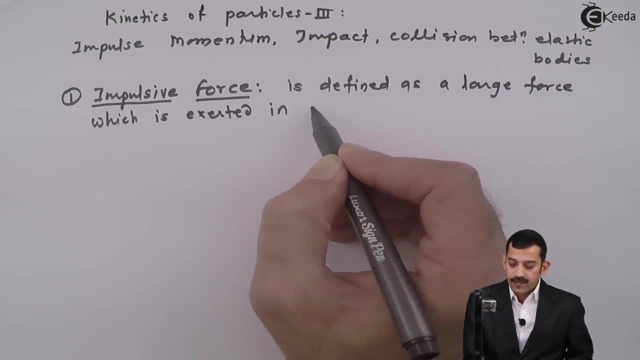 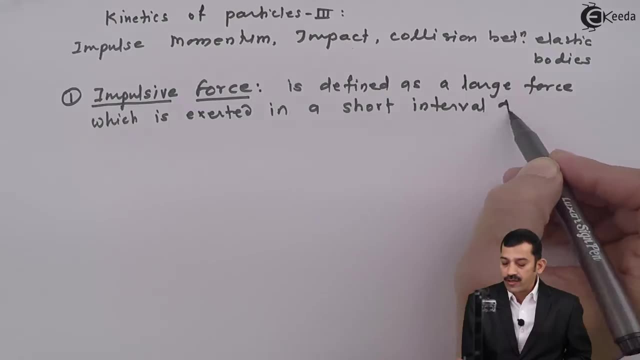 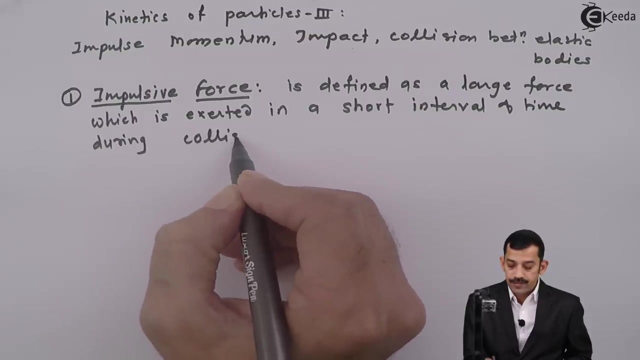 Large force in a short interval of time. in a short interval of time during collision or during collision, when such large amount of force is developed in a short interval of time, then that type of collision is called as an impact. that means impact is a particular type. 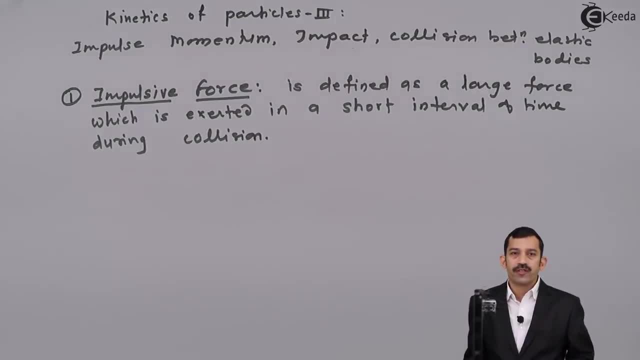 of collision, in which, when bodies collides with each other in a short interval of time, when large force is exerted, then such type of collision is called as impact. that means what these forces develop is nothing. but during collision means during impact the impulsive force is a large. 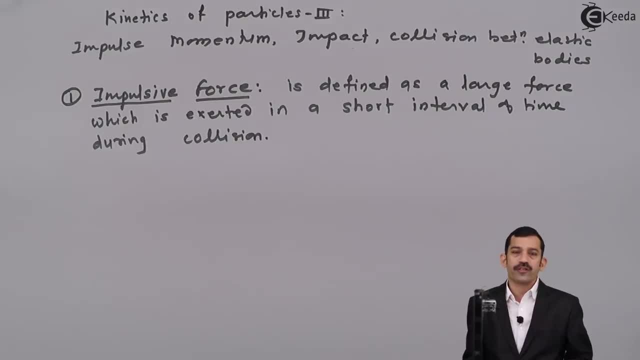 force: large amount of force which is developed in a short interval of time during collision. next term, what is important is nothing but impulse, impulse of force. now, impulse of force is nothing but simple. it is a product of these two terms. it is a product of impulsive force. what is? 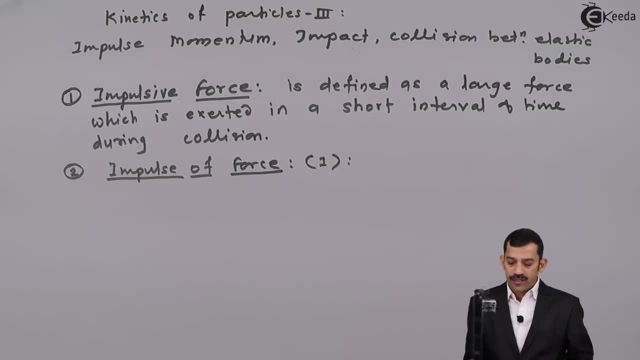 developed and the time interval in which this force acts. if we will assume the time interval in which this force acts is, say, dt or delta t, then this impulse is given by product of what impulsive force? product of impulsive force into the time interval, into time interval in which this force acts, say impulsive force is f into. 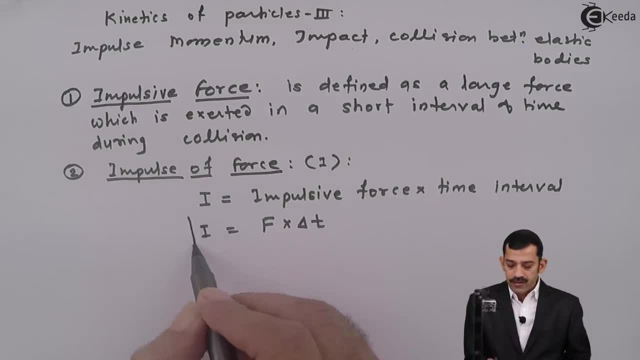 what this time interval, delta t, is nothing but impulse of a force. so first one is impulsive force term. what we have discussed is impulse of a force. number three, third term, important, what you must know here is nothing but momentum, where momentum is always a product of mass of a particular body. 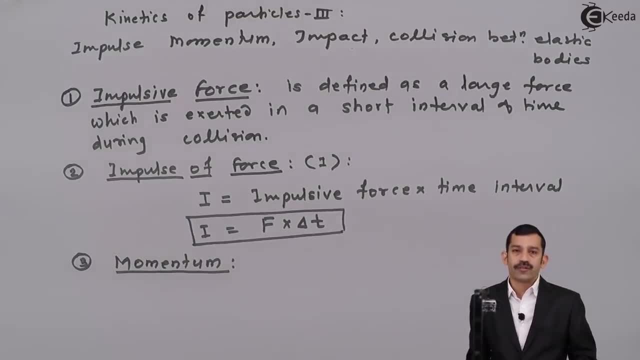 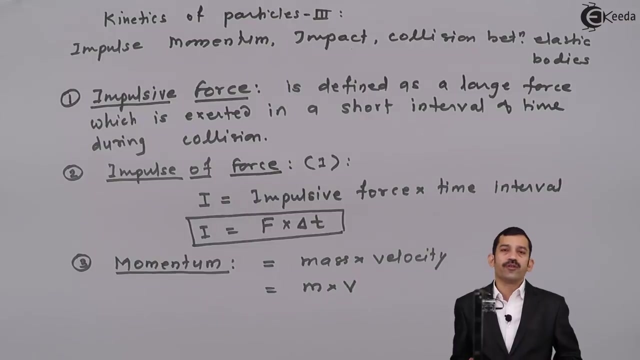 which is in motion and its velocity. that means momentum is simple, it is given by product of mass and velocity of the body. that means this one is simple: mass into what velocity? product of mass and with what velocity that particular body is moving, its velocity, where this one is a vector. 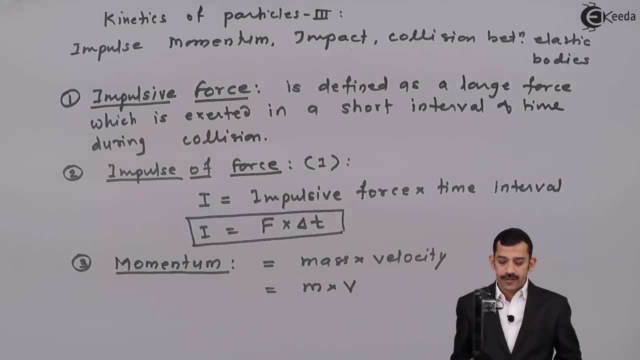 quantity depending on velocity, will substitute your values. if velocity rightward, will substitute with positive sign, velocity leftward will substitute with minus sign, if velocity is upward will substitute with positive sign and if it is in downward direction, then it is negative. that means same sign convention, what you are following in full statics as well as dynamics. 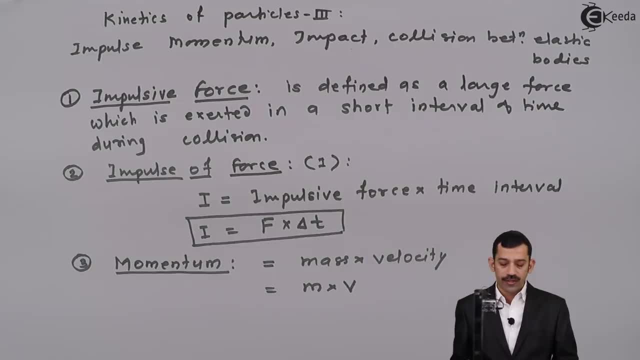 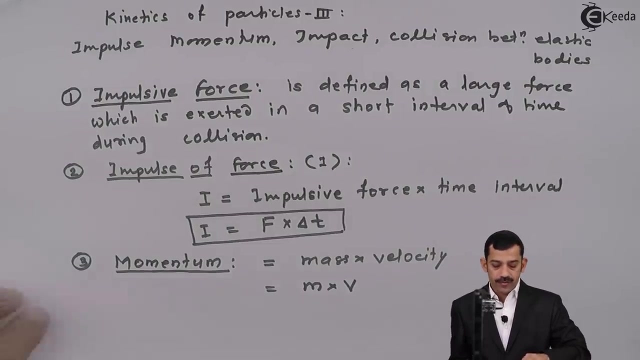 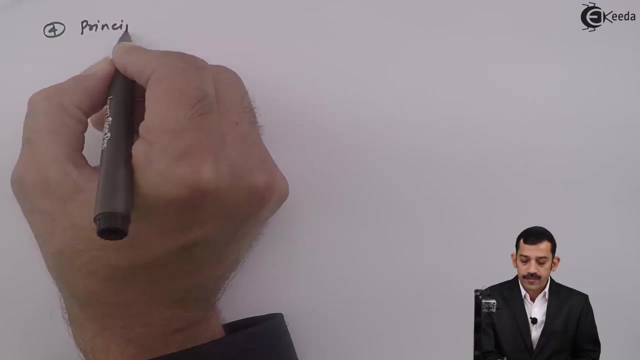 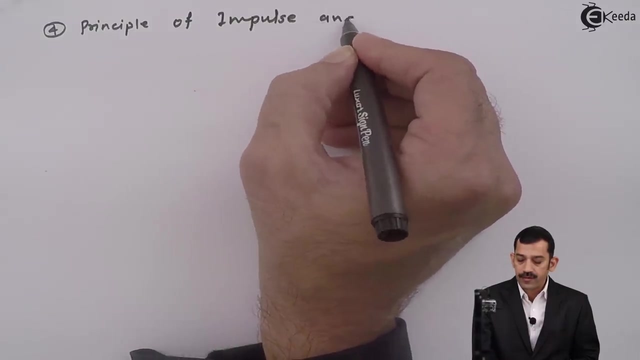 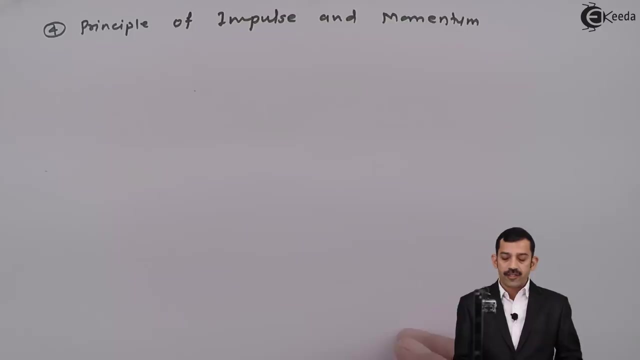 rightward positive, upward positive, leftward negative, downward negative. first term is impulsive force, second one is impulse of force and third term. what we discuss is what momentum? let's see. next part is what? fourth term, number four, principal of principal law, impulse and momentum, principle of impulse, momentum, basically relation between impulse of force and 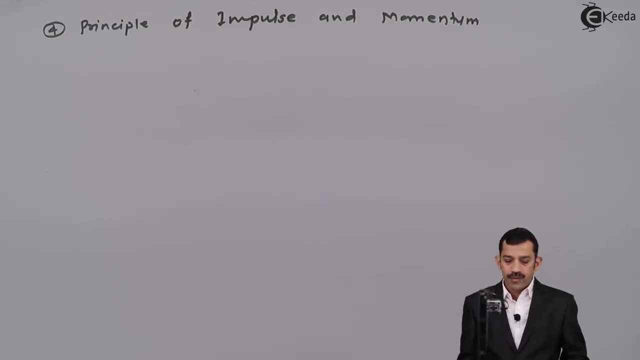 momentum in principle of impulse and momentum, which is relation between and momentum. and we will get this relation- that means principle- from newton's second law, where newton's second law is what f equal to mass, into acceleration, where f represents resultant force acting on any body, mass represent mass of body and a represents what acceleration. now, if 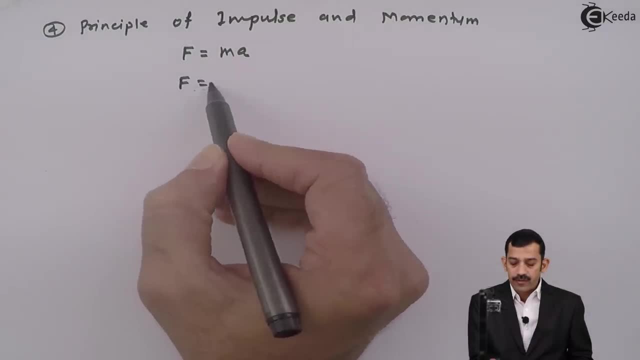 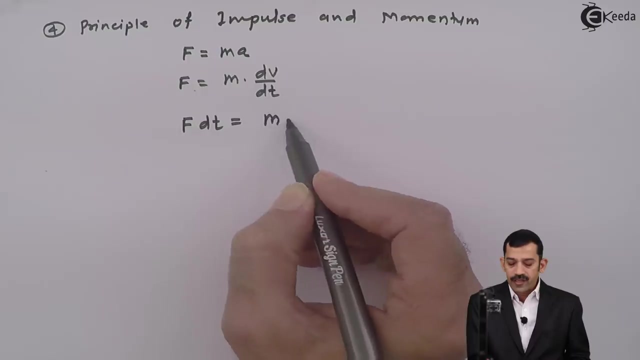 we will write this again: f equal to mass into dv by dt. acceleration is rate of change of velocity with respect to time. therefore, what we will get here- f dt equal to say m dv, now what it represents when force acts for a time interval: say dt, then velocity of body increases by dv. now, if you 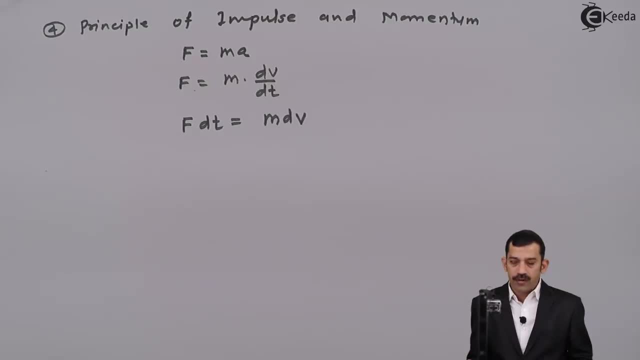 to find out that in what time interval may be from t1 to t2. what are the change in velocities? if we integrate this equation, the? what will get integral of f, dt equal to integral of m, dv, say: when time is t1, velocity of that particular mass is v1. when time is t2, velocity is, say, v2. 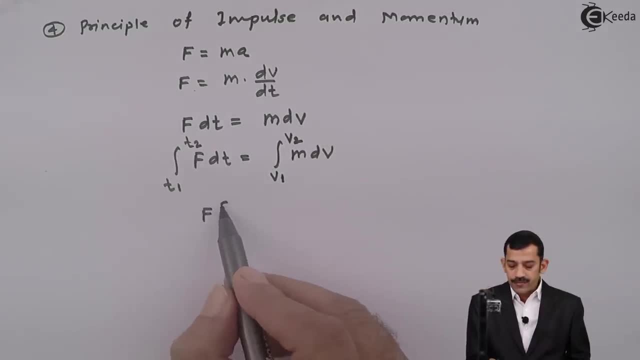 now if you integrate, what will get here? f. integral of dt is a t, lower limit is t1. upper limit is t2, equal to. integral of dv is v and mass remains constant. velocity varies from v1 to v2. that means f. this one upper limit minus lower limit means t2 minus t1, equal to. 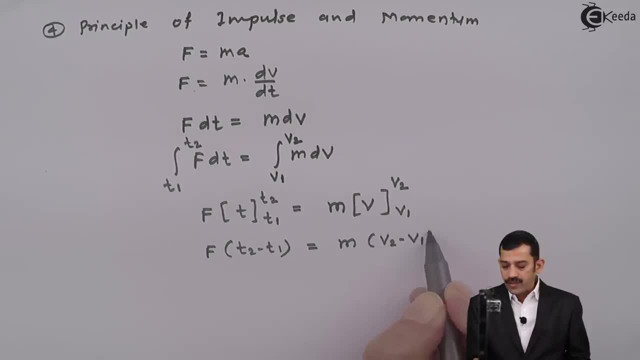 m. what will get here? f? integral of dt is a t. lower limit is t2. equal to integral of dv is v. and what will get here? v2 minus v1, upper limit minus lower limit. that means what you are getting on this left side is f into t2 minus t1 is the time interval in which force acts. 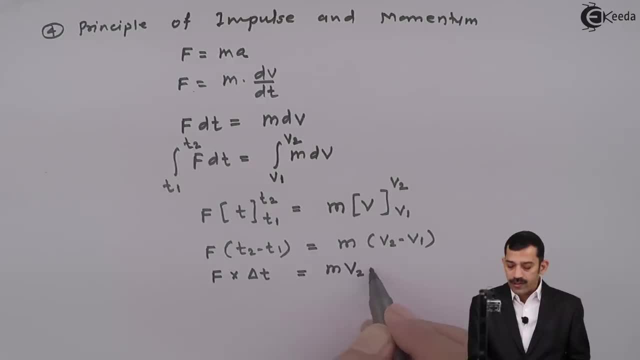 equal to. i will write this one as mv2, minus this one as mv1. as we have discussed, f into delta. t represents impulse of a force. mass into velocity is momentum. now what you are getting m into v2. v2 is a final velocity of that mass. therefore m into v2 is called as final. 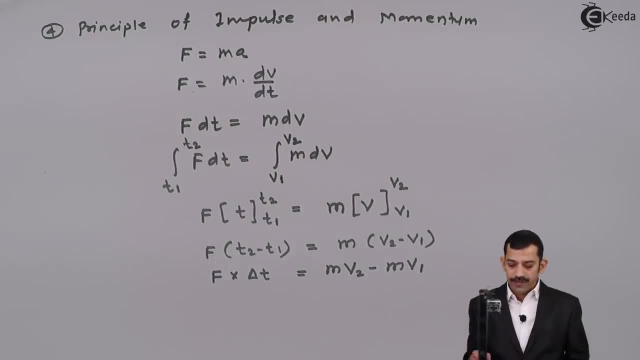 momentum m into v1 is initial momentum, f into delta, t is impulse of a force. therefore, what will get this relation as what? impulse equal to mv2 means final momentum and mv1 is initial momentum, which is relation between impulse and momentum. therefore, this principle is called, as in real, principle, of impulse and momentum. so impulse is always. 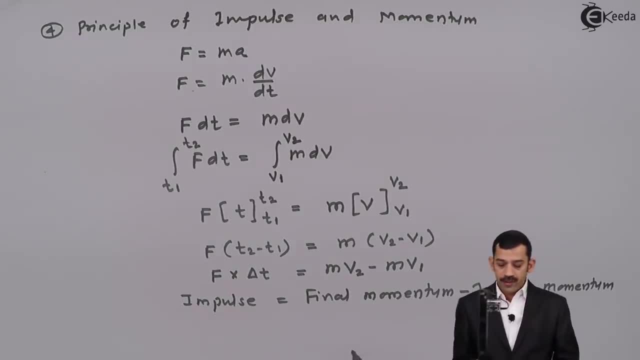 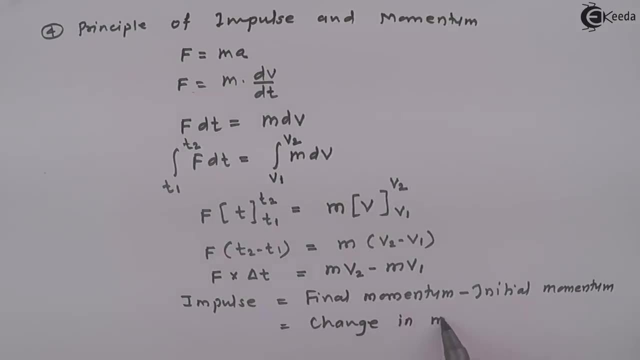 given by what final momentum minus initial momentum. this may be written as what may be. this is called as what final minus initial momentum. this is called as change in momentum. change in momentum is nothing but impulse over force. i that means in short, if you want to write, i means impulse equal to what change in momentum. 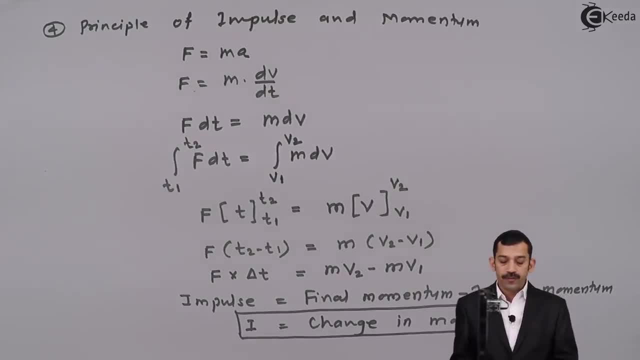 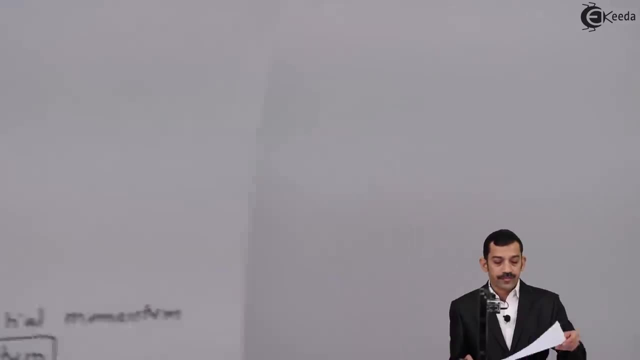 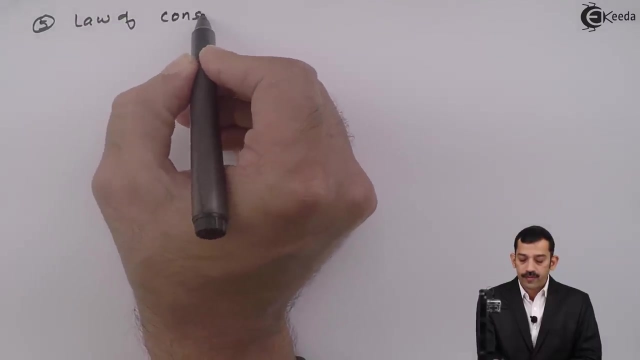 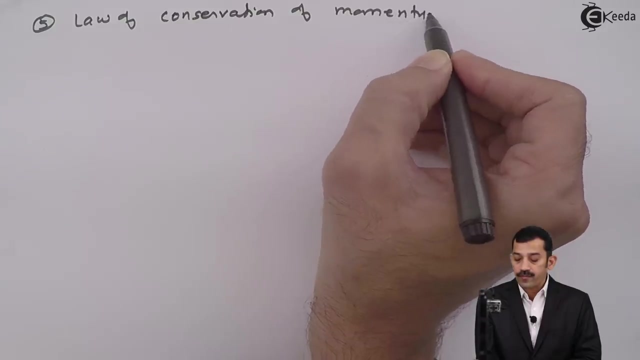 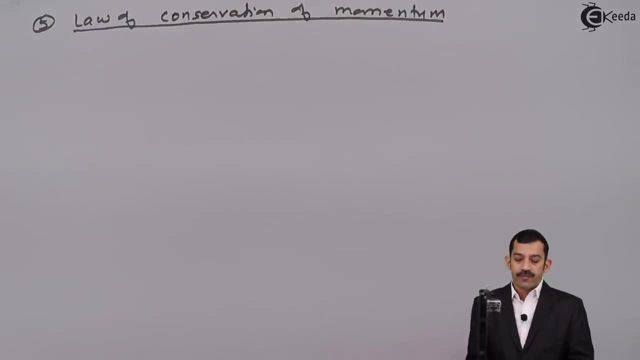 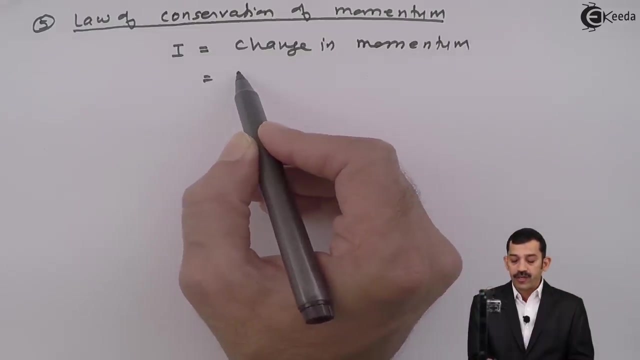 conservation of momentum, so that one will get from principle of impulse and momentum, as you know, impulse equal to what change in momentum. impulse is change in momentum. that means this one is what mv2 minus mv1 or delta mv. change in momentum is what impulse? now, when two bodies strikes with. 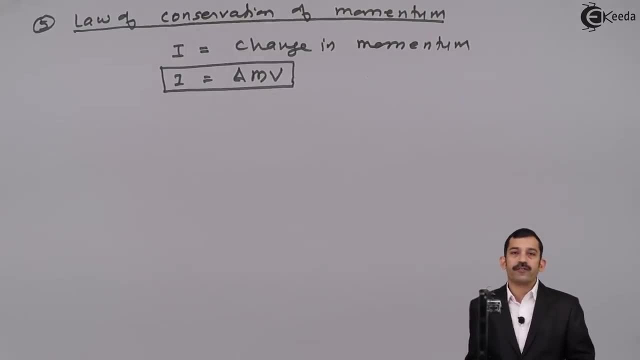 each other or collides with each other or when impact takes place, impulsive forces are developed. where magnitude of impulsive forces which are developed are same and directions of impulsive forces are opposite, as you already discussed. just see again, you, when ball strikes with bat, force is exerted by ball on the bat, say f1 to force is exerted by 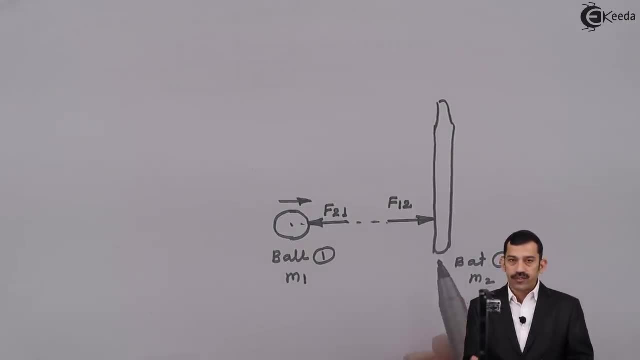 bat on the ball f2n and these forces are developed in short interval of time. that means, in this case, what forces are developed? these are developed when this ball is in contact with the bat and ball remains in contact with the bat in a short interval of time, therefore during impact. 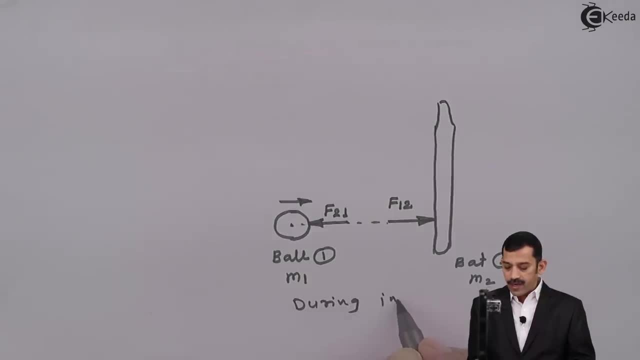 during impact. what forces are developed are a sort of reaction. therefore, magnitude of these forces are same: f1 to equal to f2n. as these forces are developed in a short interval of time, therefore, what impulse will get due to force f1 to? is f1 to into dt rightward? you can say positive. 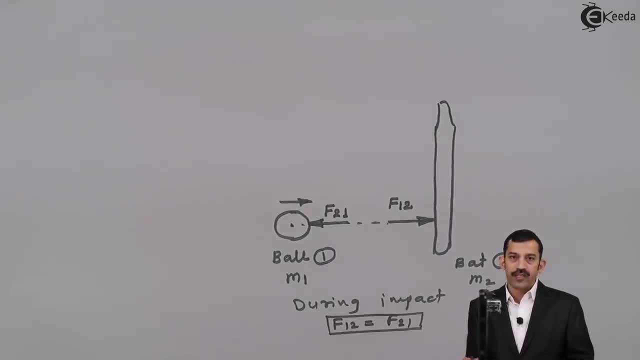 next one, f2n, into delta t, which one is in leftward direction. that means it is negative, that means during impact. if we will add these impulses of the force or sum of impulses during impact is zero, because magnitude of forces are same and directions are opposite. as sum of impulses is zero, that means 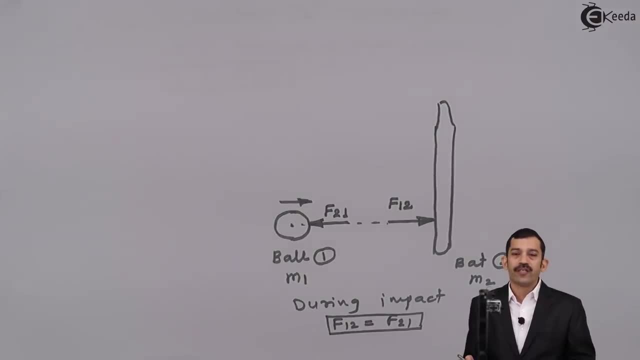 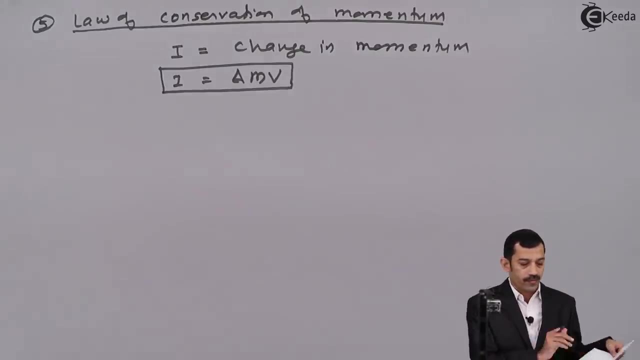 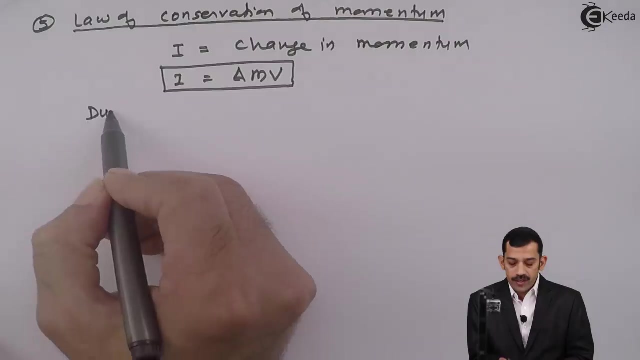 i term is zero on left hand side. so what will get here change in momentum equal to zero. therefore, what we are reading here is that if we will add these impulses of the force or sum of impulses during impact, there are some other that we have to see to fit this problem, because we have written first: recall operation. 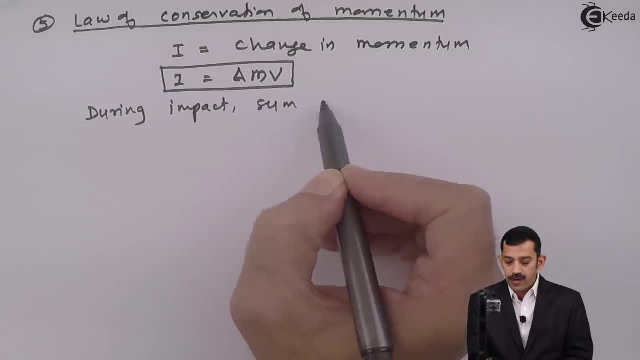 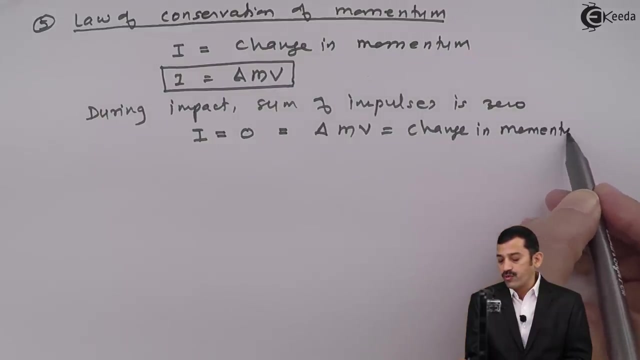 is i equal to, i is delta mv and i isant to be beaten: &i is, &i is 00. So when i is written, i is delta mv. during impact, That means change in momentum during impact. is what? 0 as a change in momentum what we? 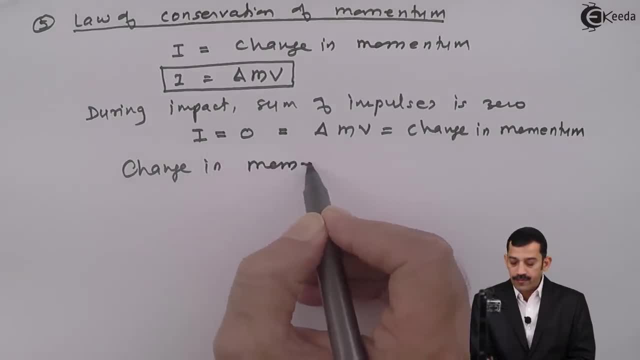 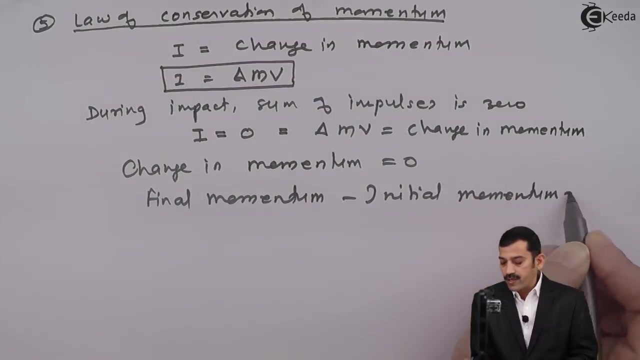 are getting finally change in momentum equal to 0. change is what? final momentum minus initial momentum? that means final momentum minus initial momentum equal to 0. final momentum minus initial momentum. final momentum minus initial momentum: 0. that means: can you say final momentum equal to initial momentum or initial momentum equal to final momentum? that means here, if I will write: 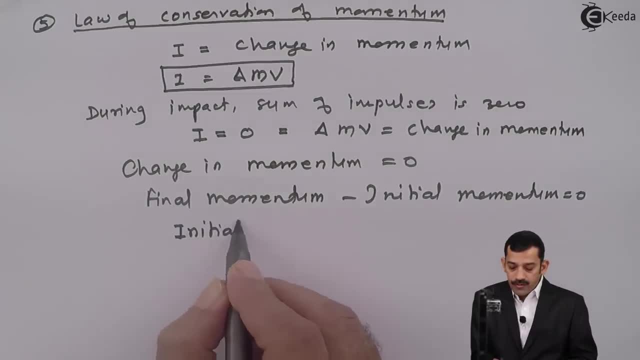 log, conservation of momentum. so it is finally what? initial momentum? initial momentum equal to what we will get here. final momentum, now this one is possible during impact. now, in impact, always two bodies are involved. say, first body is of mass m1, second body is of mass m2. 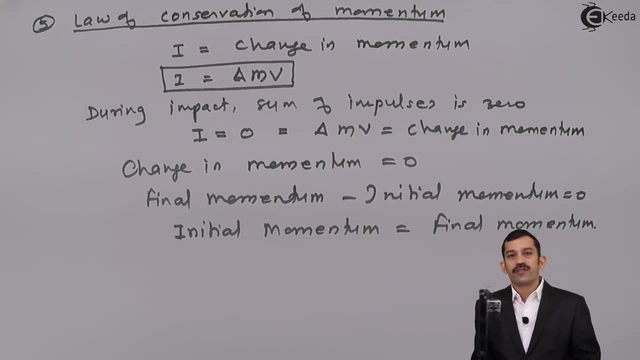 body 1 moves with some velocity v1. body 2 moves with some velocity v2. so initial momentum is mass into velocity of each body. so for first body initial momentum is written as m1, v1 plus. for second body it is written as m2- v2. 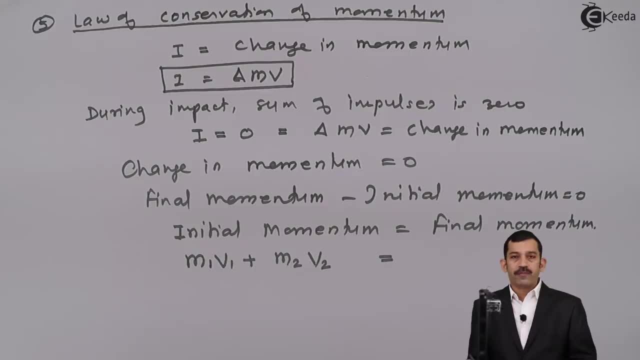 which is equal to final momentum, is after impact. what is the momentum now after impact? velocities of bodies changes. therefore, here final momentum of first body, will write m1- v1 dash, and for second body I will write this one as m2- v2 dash, where v1 dash and v2 dash are velocities of bodies 1 and 2. 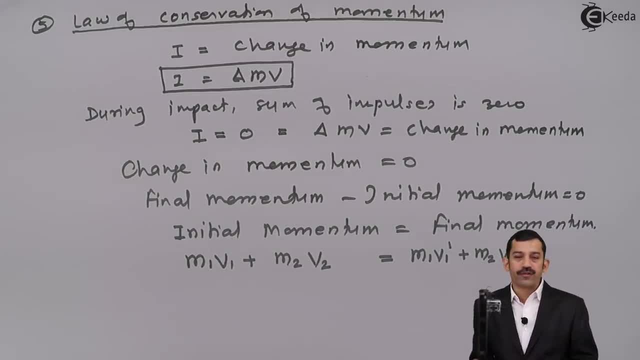 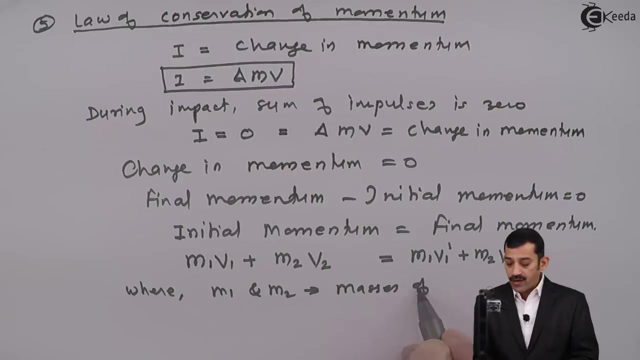 just after impact. m, v1 and v2. these are velocities of body just before impact. m1 and m2 are what masses of bodies 1 and 2 which are involved in impact. therefore, here these terms represents what m1 and m2 masses of bodies 1 and 2 respectively. v1 and v2 represents what velocities of bodies 1 and 2 respectively. 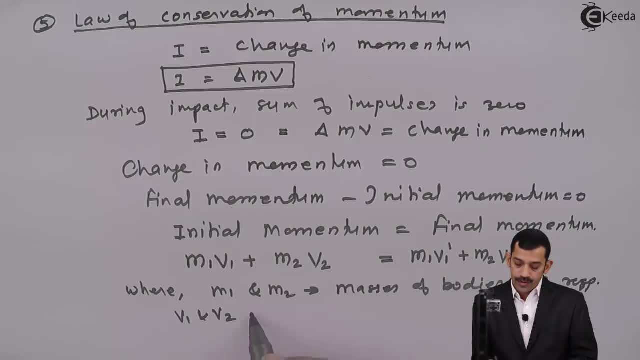 vs and v2 represents what velocity's of bodies, 1 and 2 respectively. 1 and 2 is placed in volt, absolute velocity relative to credit defective current content. Och we all know that V1, V2 represent what velocity of bodies and velocity of the JUDXed in theетр 어떻y of second body var game world. and we know that we are the same as percasso. MCX is also the same as before. we are not the same as the previous cards. 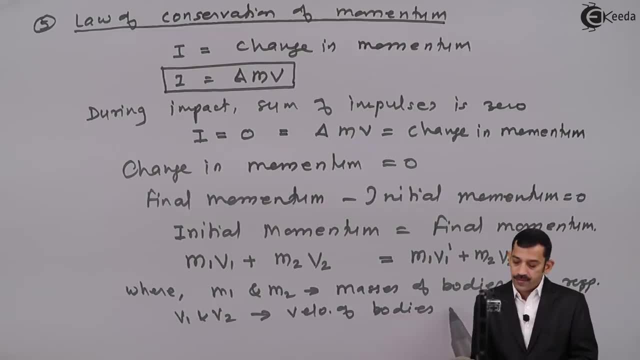 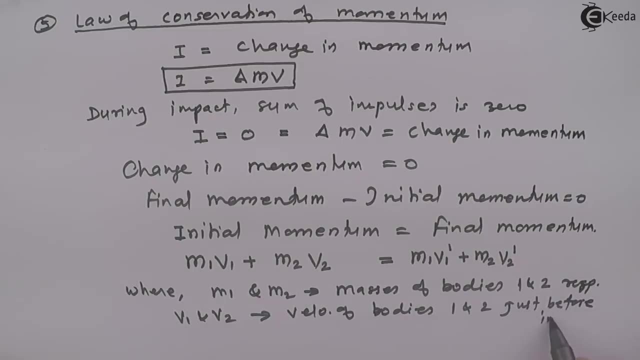 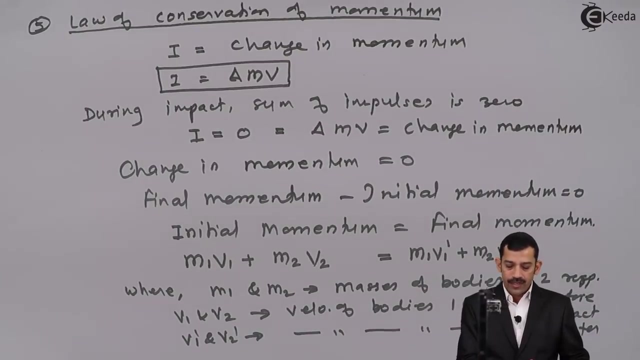 of bodies, one and two just before impact. v1- dash and v2 dash represent velocities of bodies, one and two just after impact. just after impact in law of conservation of momentum. finally, what we are getting: m1 v1 plus m2- v2, equal to m1- v1 dash plus m2- v2 dash, where m1 and m2 represent masses of. 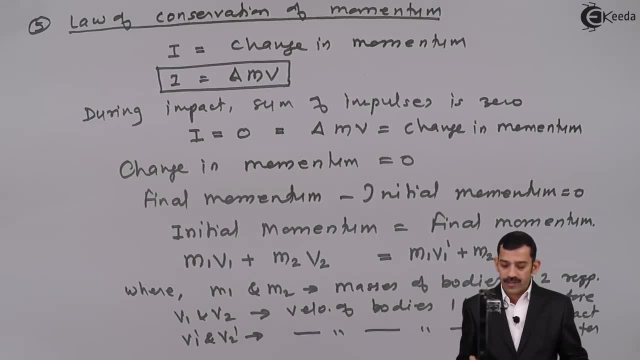 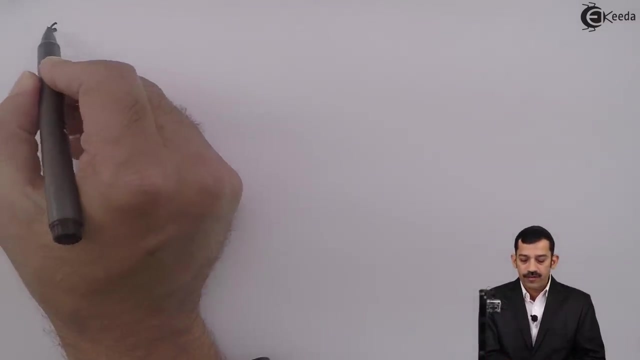 bodies one and two respectively. v1 and v2 represents velocities of bodies one and two just before impact. v1- dash and v2. dash represents what velocities of bodies one and two just after impact. next term, again, we will discuss now. next important term is coefficient of restitution, coefficient of 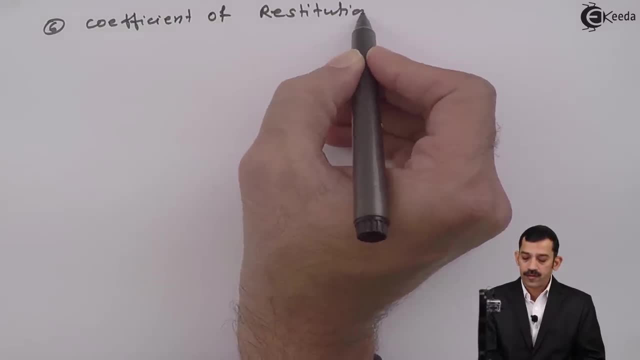 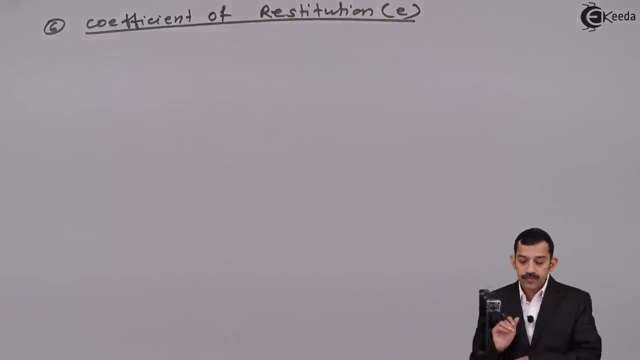 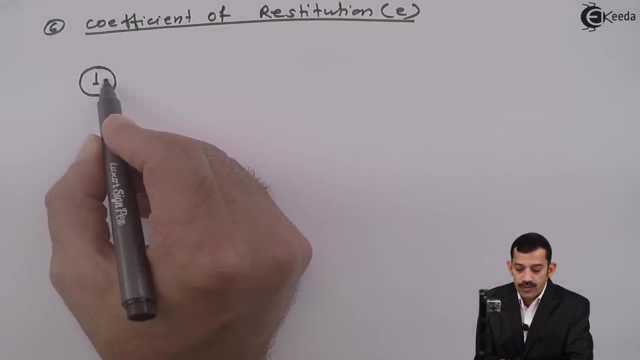 restitution and is represented by e. now, coefficient of restitution means what for that one, just here, if say this one is one body of some mass, m1 say body one, its mass is m1, and this body moves in rightward direction with velocity v1, that means first body. 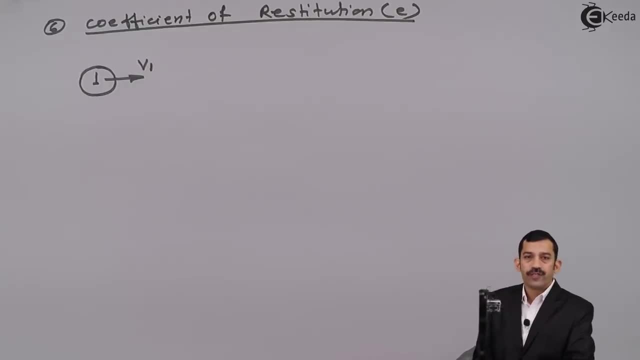 one of mass m1, moves in rightward direction with some velocity: v1. similarly, there is one more body, say body two, of mass m2, which one again moves in rightward direction. save it, that means both the bodies are moving in same direction. and if i'll say body one strikes, 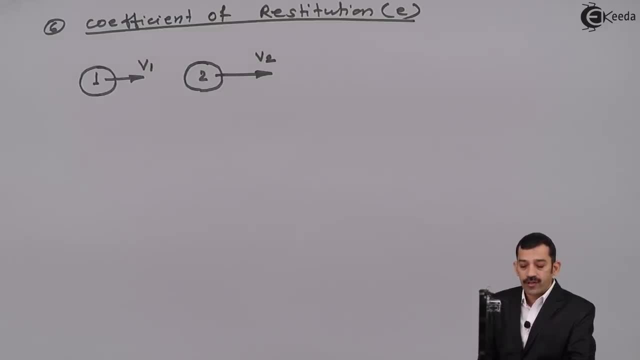 with body two. if body one strikes with body two, then velocity of body one must be greater than velocity of body two. then only body one strikes with body two, or you can say collision takes place or impact takes place. that means for this collision velocity of body one must be greater than velocity of body two, then body one strikes with body two. 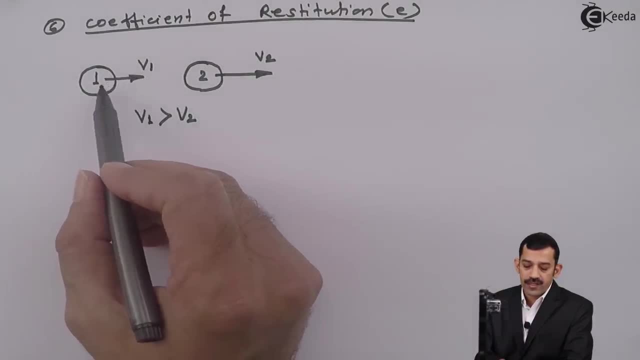 as velocity of body one is greater and as time passes say initially they are at some particular distance. as time passes the distance between the two bodies gradually decreases and finally body 1 strikes with body 2. that means what you can say: body 1 approaches towards body 2 before impact. therefore, this difference in velocity- if you take here v1- 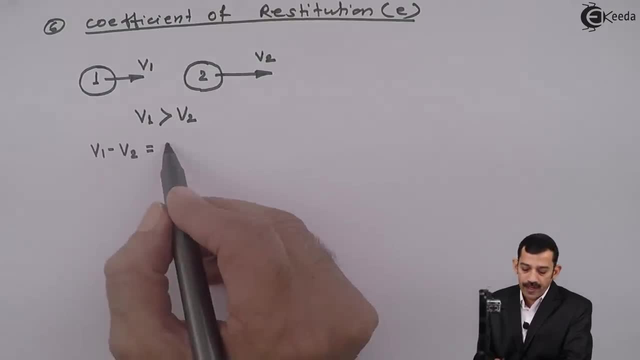 minus v2 will get positive value because v1 is greater and this velocity is called as velocity of approach. is called as velocity of approach. so before impact difference between the velocities of these two bodies, v1 minus v2, is velocity of approach, because body 1 approaches towards body. 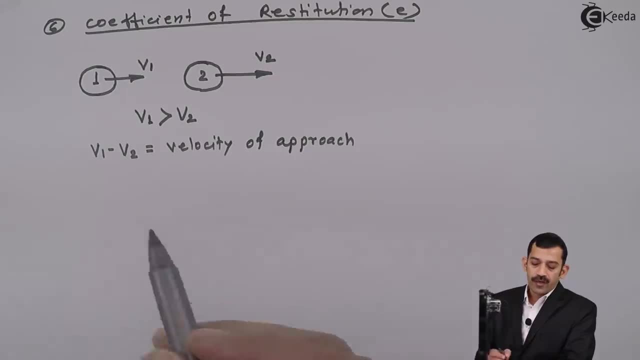 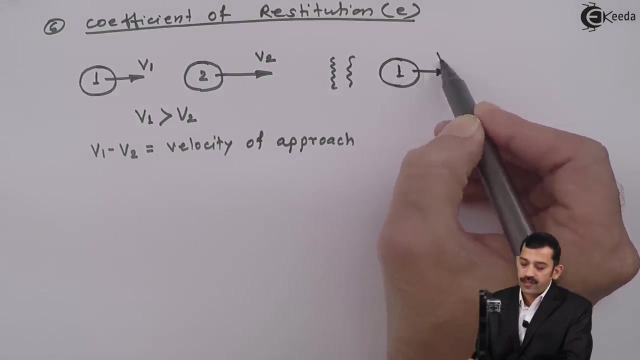 2 as v1 is greater than v2. when body 1 approaches and finally say body 1 strikes with body 2, say this one is the impact. once body 1 strikes with body 2, what happens? this body 1 actually moves with some velocity after impact. say v1 dash just after impact. velocity of body 1: v1 dash. 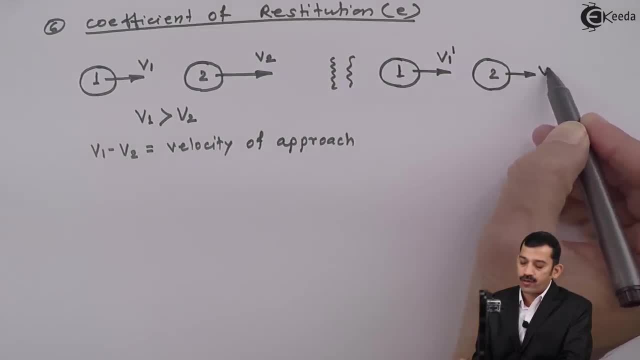 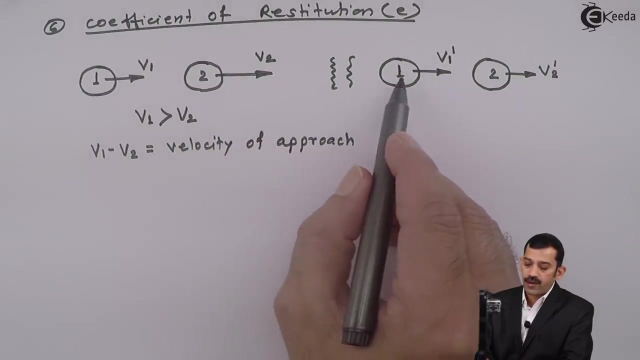 and just after impact. velocity of body 2 is what v2 dash, v1 dash and v2 dash represents: velocities of bodies 1 and 2 just after impact. that means after impact, as bodies separates with different velocity. definitely velocity of this body 2 must be. 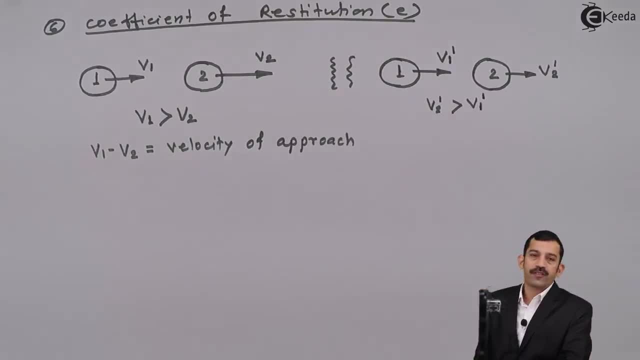 greater than velocity of body 1, then only you can say: separation is possible. otherwise bodies can't separate from each other. if, for example, if you will assume v1 dash is greater and v2 dash is less, then separation is not possible. what happens? body 1 pushes body 2 in rightward direction, as 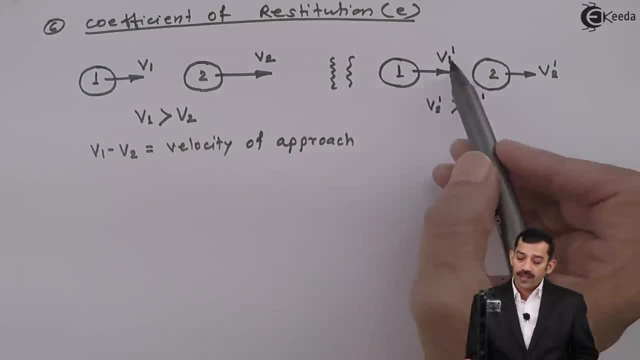 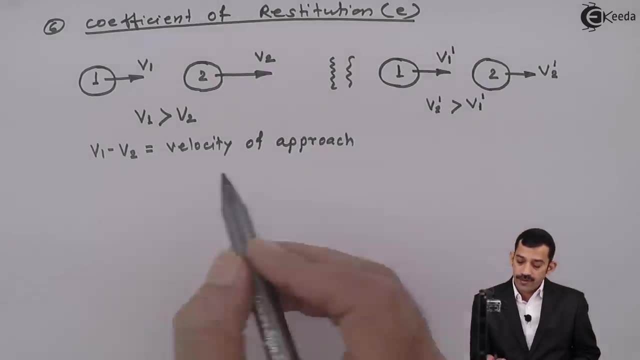 velocity is greater. if velocity of body 1 is greater than velocity of body 2, then separation is not possible. if velocity of body 2 is greater, less and velocity of body 2 is greater, then only separation is possible. therefore, what difference in velocity you will get between v2 dash and v1 dash? this difference is positive and is called 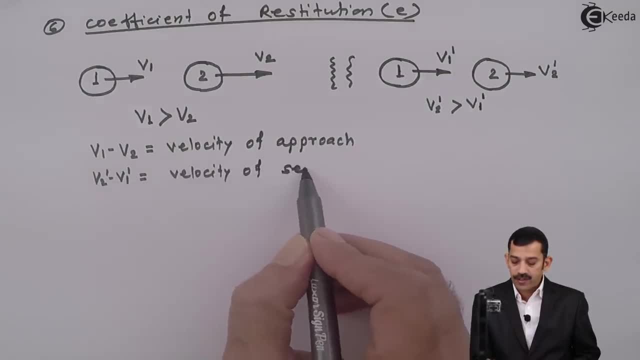 as what velocity of separation and is called as velocity of separation. now, depending on these two bodies which are given, that maybe you can say glass marble, this one is also glass marble, maybe this one is plastic, this one is plastic, this may be plastic and maybe glass marble. 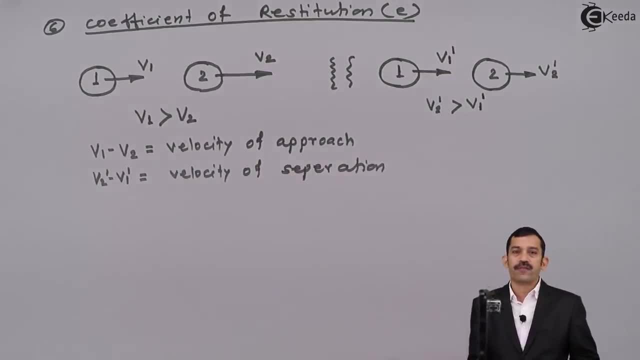 may be plastic and maybe wood, any pair of material. if we take any pair of material during collision, whatever be the two bodies collides with each other, or any particular type of pair. any two materials are involved or materials may be same. mL 2 is echocשה. 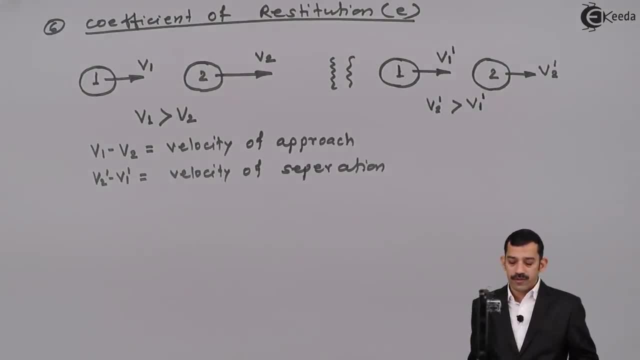 This ratio of velocity of separation to the velocity of approach always remains constant and is called as coefficient of restitution. That means how we will define this term: coefficient of restitution. The coefficient of restitution is defined as the ratio of velocity of separation to the velocity of approach. 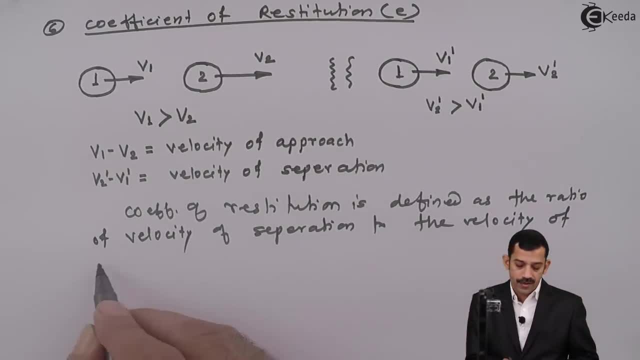 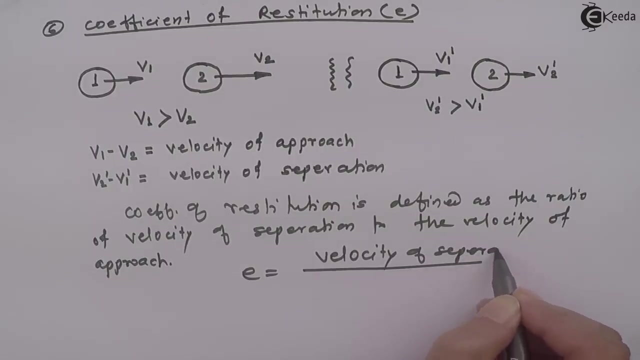 The velocity of approach to the velocity of approach. That means, if we will write this coefficient of restitution as E equal to so what we will get here? Velocity of separation to the velocity of approach. Let's continue on next page. Velocity of separation to the velocity of approach. 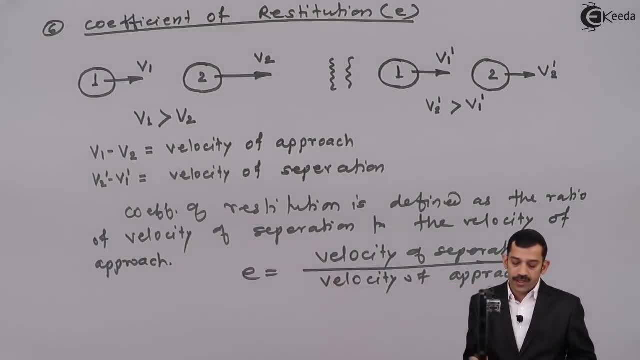 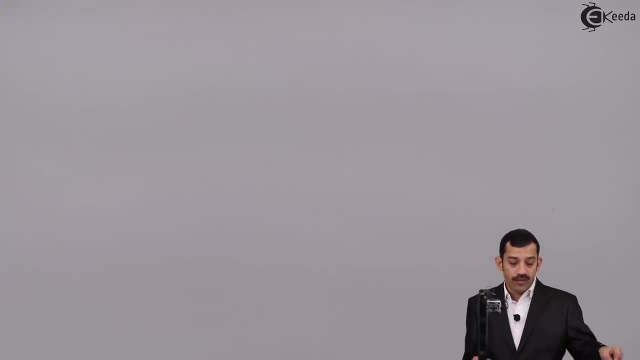 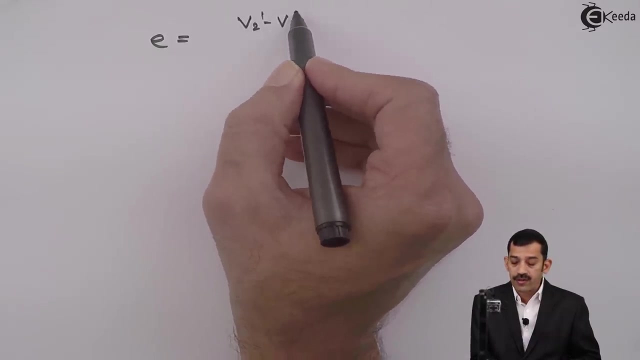 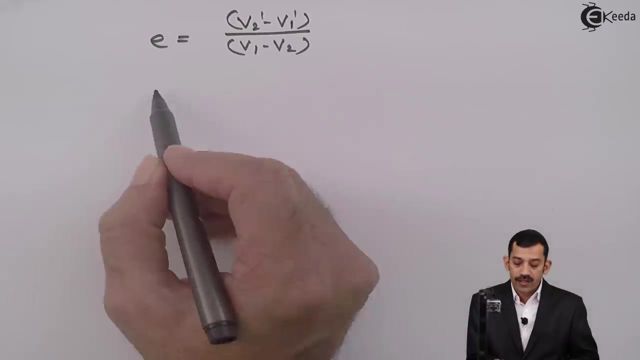 Velocity of separation to the velocity of approach. Velocity of separation. You know, velocity of separation is V2 dash minus V1 dash. Velocity of approach is V1 minus V2.. We will substitute these values here. E equal to velocity of separation is V2 dash minus V1 dash, and velocity of approach is V1 minus V2.. This one may be written as if I will take minus sign common from denominator. it becomes V2 dash minus V1 dash. 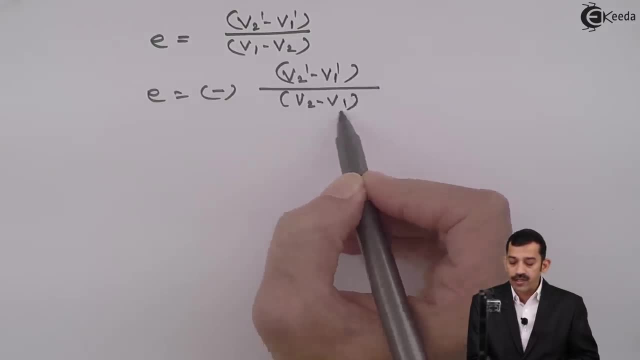 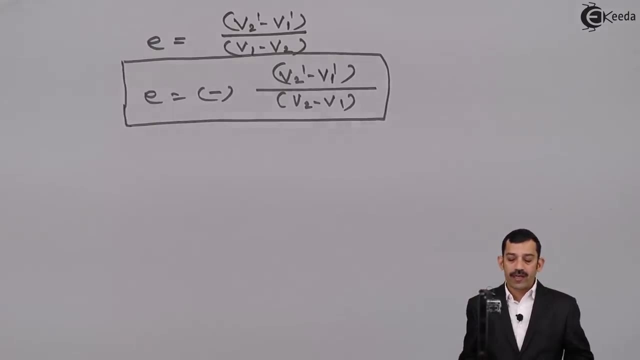 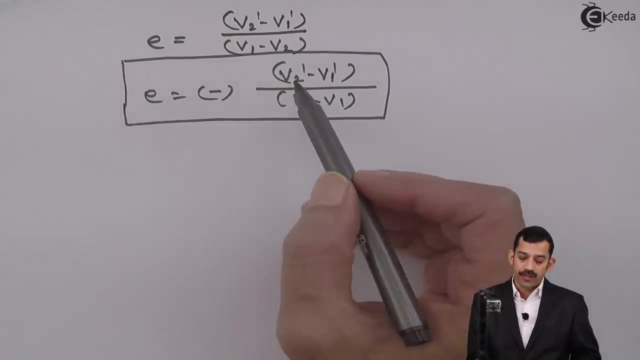 V2 dash minus V1, dash upon V2 minus V1.. If we will write like this, then this recalling formula becomes easy. The coefficient of restitution is given by minus of V2, dash minus V1, dash upon V2 minus V1.. That means first velocity, always for second body. Second, what we are subtracting is velocity of first body and in numerator velocities of bodies after impact, in denominator velocities of bodies before impact. 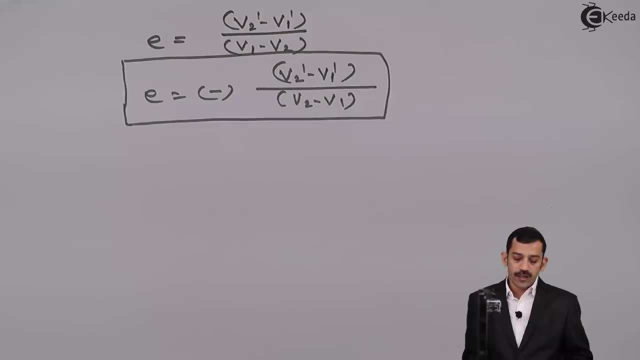 And complete value is with minus sign. Now, depending on value of this, E, coefficient of restitution. E value varies from 0 to 1.. Range of coefficient of restitution is 0 to 1. Depending on what value of E is given. accordingly, these collision between the bodies or impact. they are divided in three categories. Therefore, we will write this one as what point number 7.. 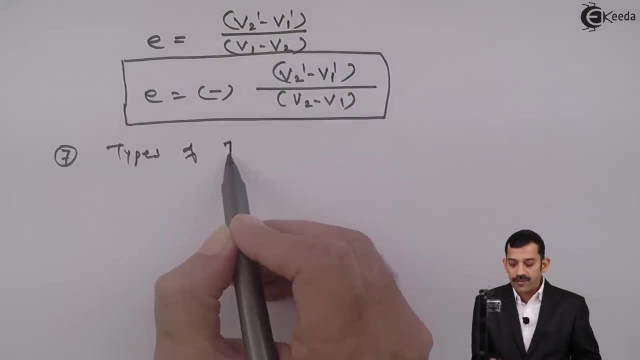 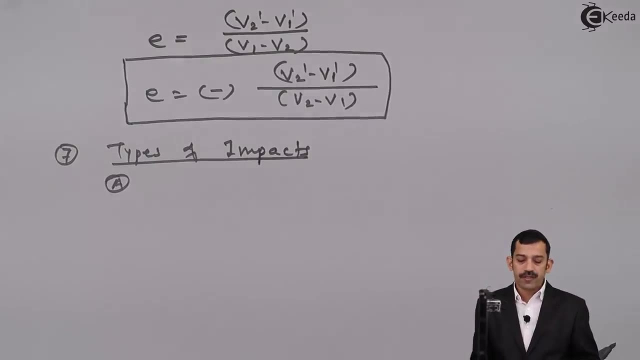 Say from this one what will get types of impacts In that one number: 1. That means first case. you can say 8. If E equal to 1. That means if coefficient of restitution equal to 1., Then the impact. Then the impact is called as E equal to 1.. 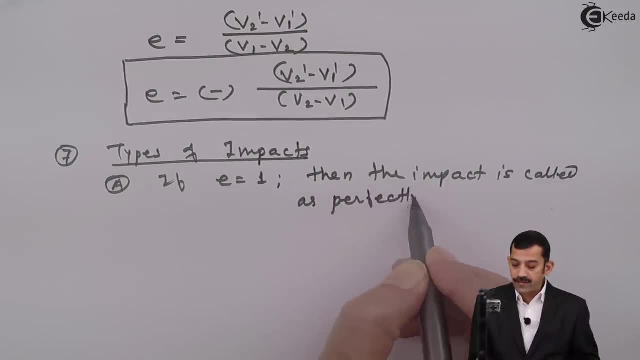 perfectly elastic impact. So may be in some problem. E value is not given as 1 and in wording may be written: coefficient of restitution is not 1.. What is given When two bodies collides with each other, assuming, say, impact is perfectly elastic? Whenever this wording is given, E 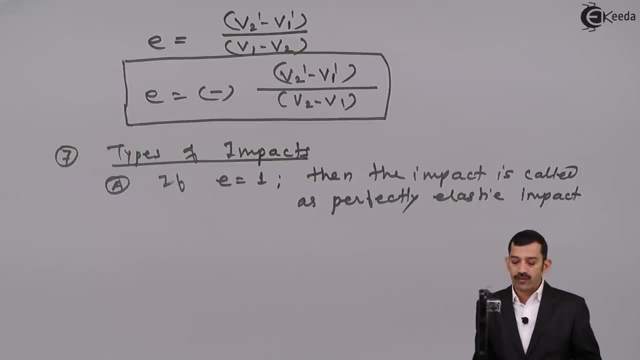 is not given, then what we will do? We will take E equal to 1 for perfectly elastic impact, because when E equal to 1, then the impact is called as perfectly elastic impact. Then value of E may be. you can say E, what you are getting is less than 1 and is greater. 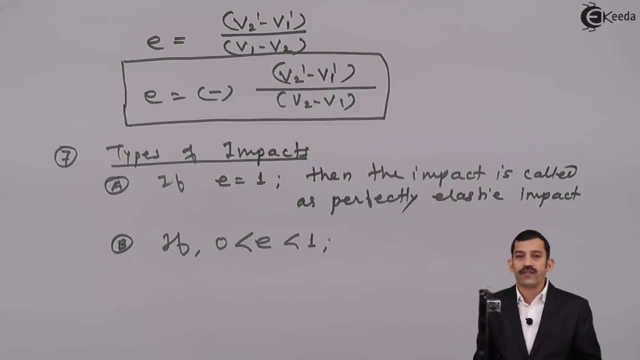 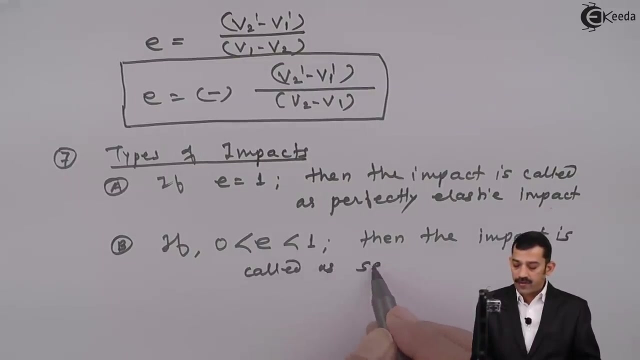 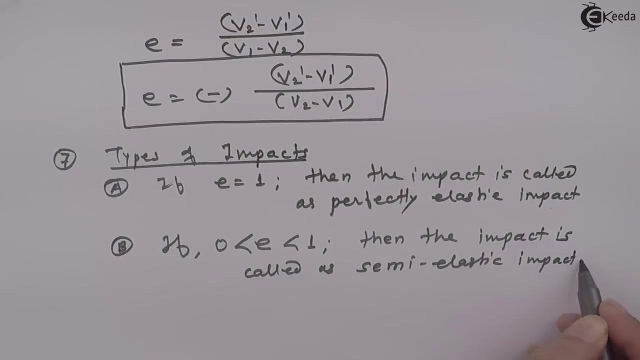 than 0.. Any value between 0 and 1, greater than 0 and less than 1. if such value is given, then the impact will be less than 0. Then the impact is called as semi-elastic impact. Then it is called as semi-elastic. 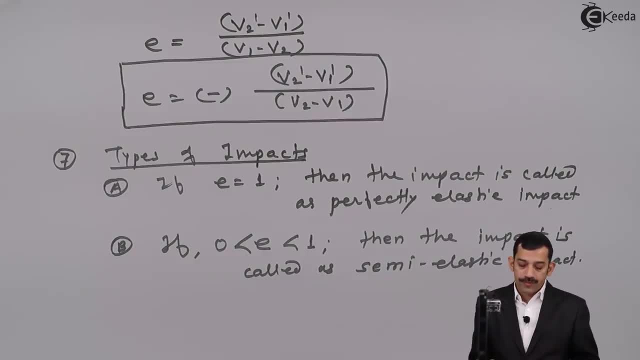 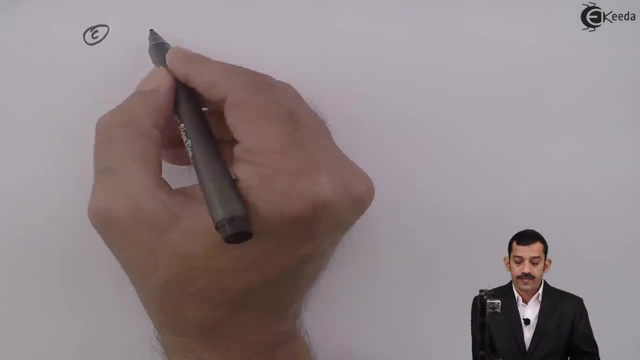 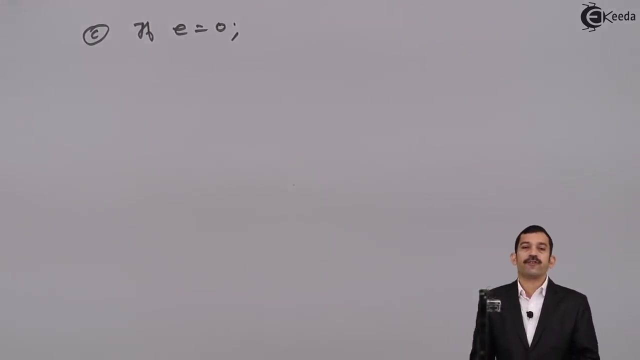 impact. Again, what is possible? Third case: you can say: see if E equal to 0.. If E equal to 0- this one is also possible. When E equal to 1, impact is perfectly elastic. impact E is greater than 0, less than 1 impact. 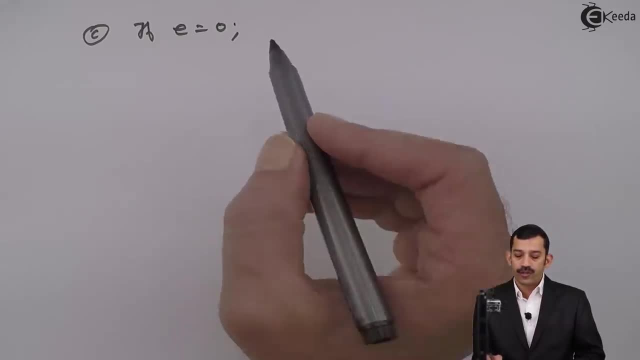 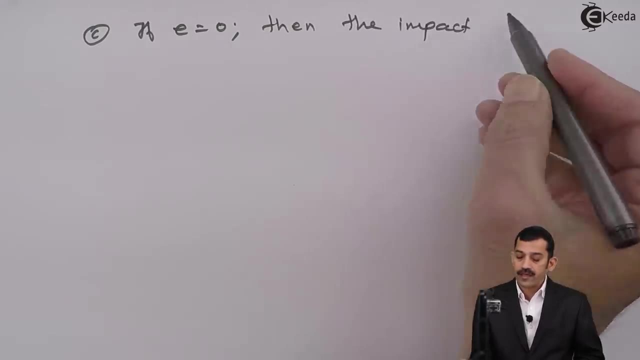 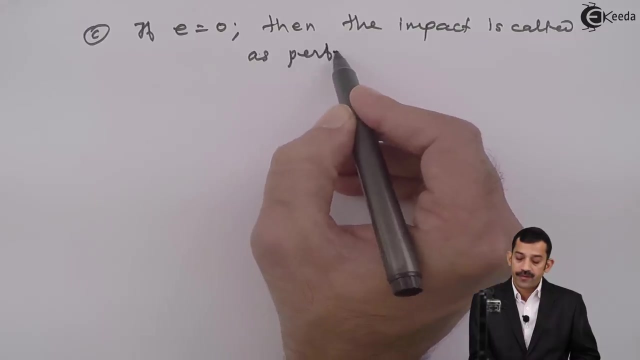 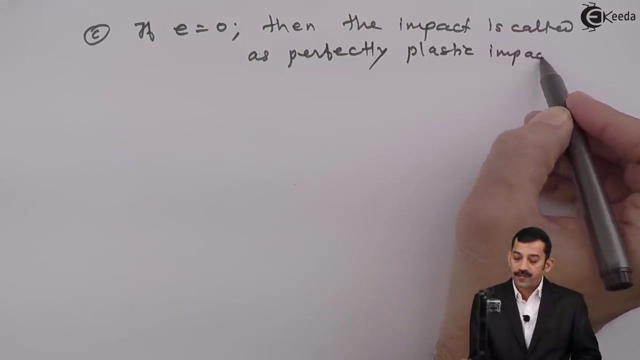 is called as semi-elastic impact. If E equal to 0, then the impact is called as, then the impact is called as perfectly plastic impact. Perfectly plastic impact: That means from range of values of E, you will get some three different types of impacts. 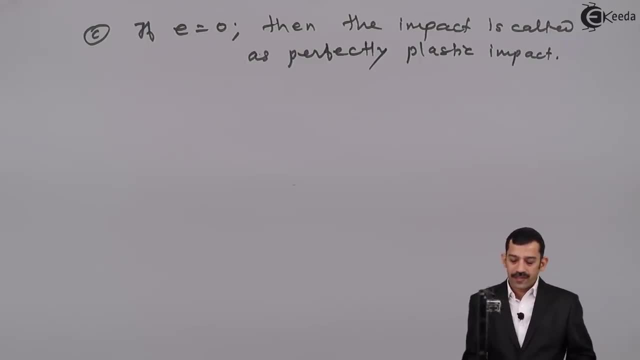 When E equal to 0, impact is perfectly plastic. Now, if you will substitute value of E as 0 in our formula, Our formula of E is what V2 dash minus V1 dash upon V2 minus V1, and which is equal to 0.. What you are writing? This is E. You are writing E equal to 1.. So V2 dash minus V1, dash upon V2 minus V1, and which is equal to 0.. What we are writing? This is E equal to 1.. So you. 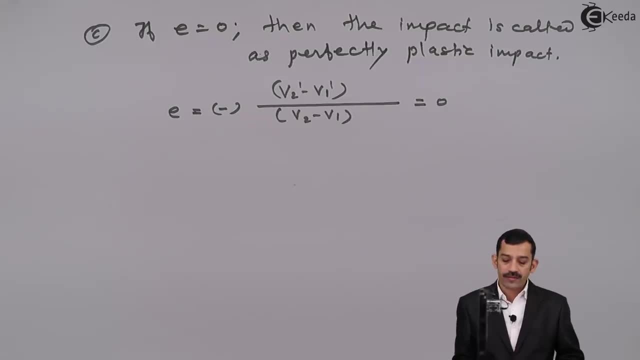 writing. this equation is for perfectly plastic impact. So for perfectly plastic impact, E equal to 0, that is minus of V2, dash minus V1, dash upon V2 minus V1, this term is 0.. If you multiply here denominator to 0, so what you will get on right hand side is what 0. 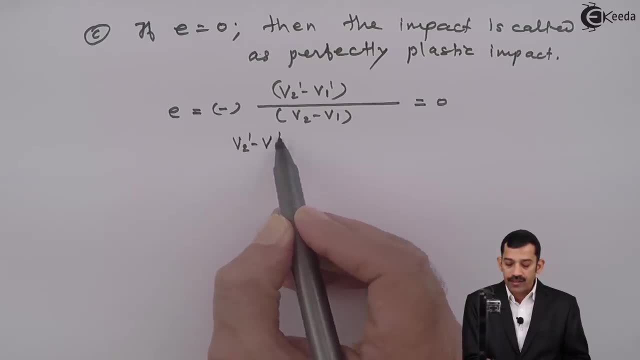 Therefore, can you say V2 dash minus V1 dash equal to 0.. Therefore, V2 dash equal to V1 dash. Now what it represents: V2 dash means velocity of body 2 just after impact. V1 dash represent velocity of body 1 just after impact. That means V2 dash equal to V1 dash. that means: 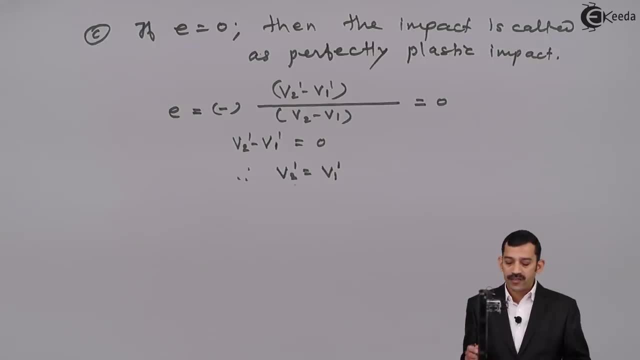 velocities of bodies 1 and 2 after impact are same. Therefore, this velocity may be written as V dash and called as what? As both the velocities are same after impact, it is called as common Velocity after impact. Is it possible to find out this magnitude of this velocity, V dash or? 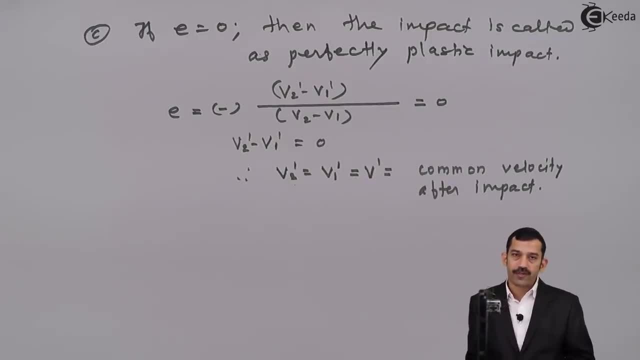 you can say V1 dash or V2 dash. that means common velocity after impact. So you know law of conservation of momentum. Law of conservation of momentum is what M1 V1 plus M2 V2, equal to M1- V1 dash plus. 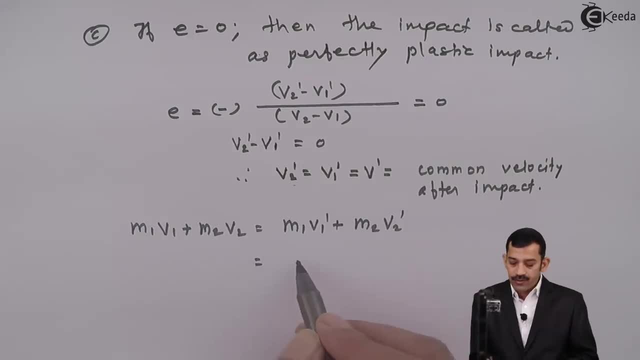 V2 dash. M2, V2 dash. As you know, V1 dash and V2 dash are same. that means I will write this one as what V dash common, because V1 dash and V2 dash is having same magnitude. That means M1, V1 plus M2. 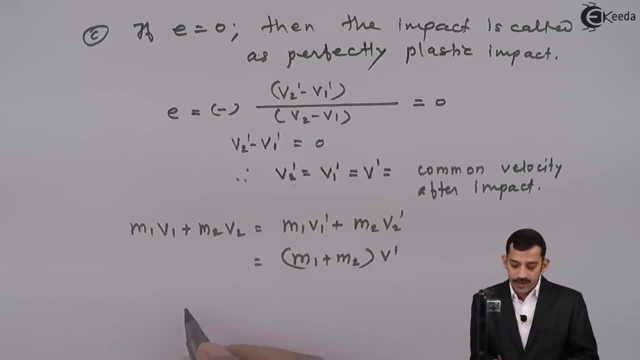 V2 equal to M1 plus M2 into V dash. that means this V dash common velocity is given by what M1 V1 plus M2 V2 upon M1 plus M2 V2.. That means this V dash common velocity is given by what M1 V1 plus M2 V2 upon M1 plus M2 V2.. 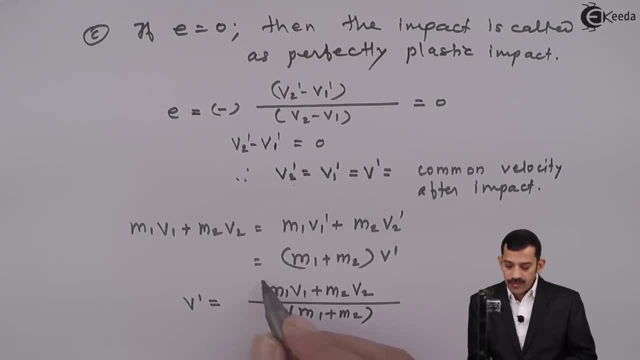 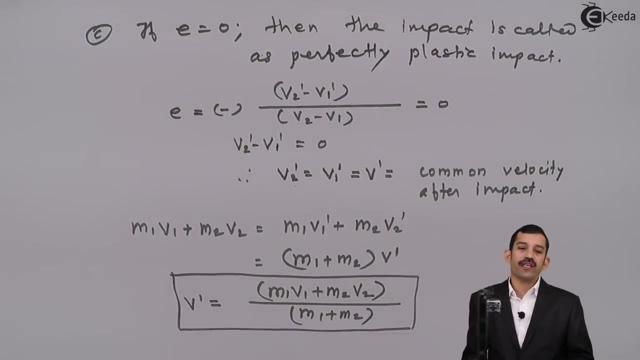 Use of this equation while solving problem. if impact is given as a perfectly plastic impact directly, we will use this V dash as what Common velocity? to find out velocity of both the bodies just after impact. You know, once we will get this coefficient of restitution and from that one 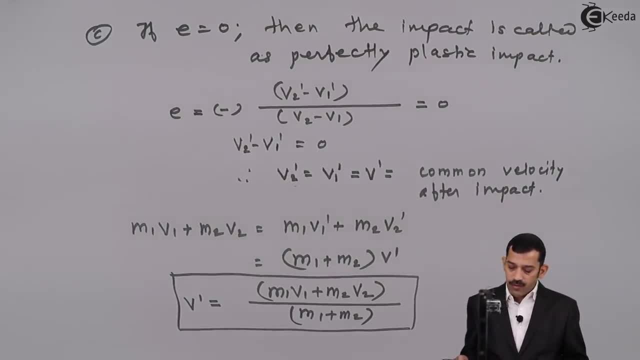 types of impact. we are getting right. One more again. some types of impact you will get depending on direction of velocities. What you are getting now, three types: perfectly elastic, perfectly plastic and semi elastic. impact from values of coefficient of restitution. Similarly, from direction of 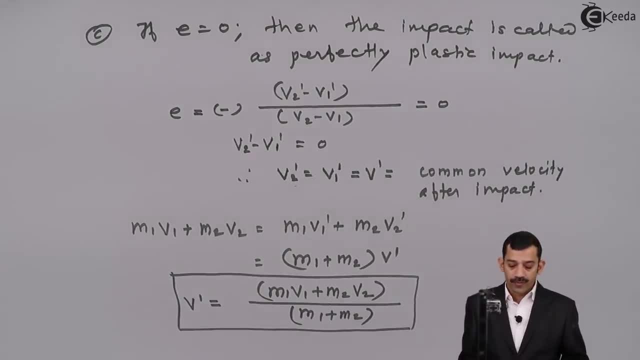 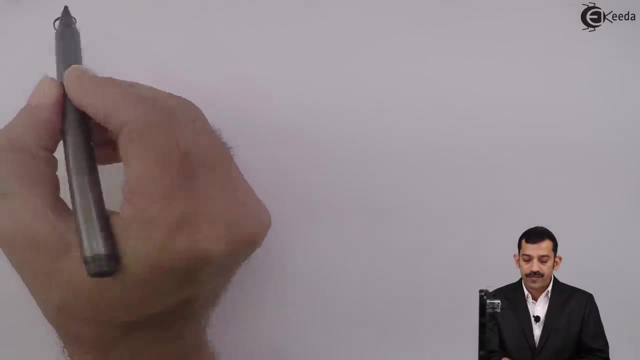 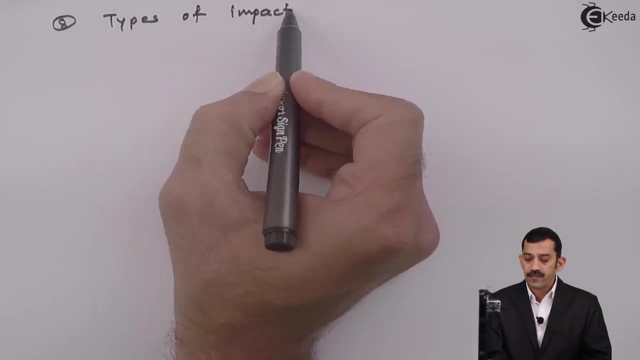 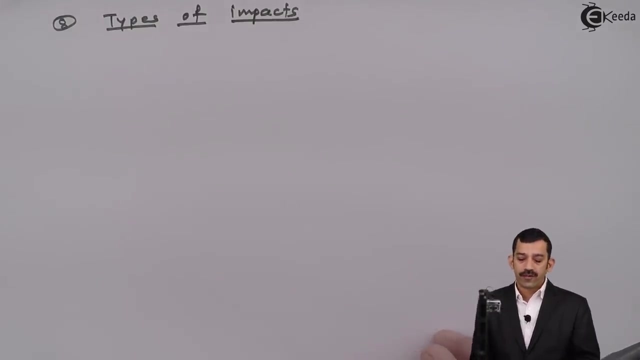 velocities also, we will get some types of impact. Therefore, next point is: what now Say point number 8. Again, I will write here types of impacts. But these types depends on what Their velocities, directions of velocities, For example, say this one is A, Now this one is, say, one body, This one is body one. Next body I will represent. 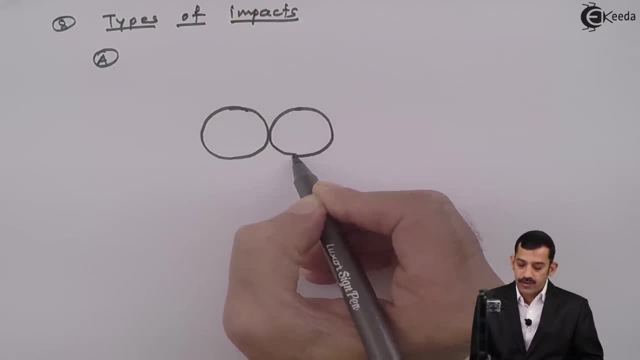 here, during impact, body two is in contact with body one, Say body one and body two. Now important point is what here, When two circular bodies are in contact with each other, first we will identify contact point. Contact point is this point where two bodies are in contact. 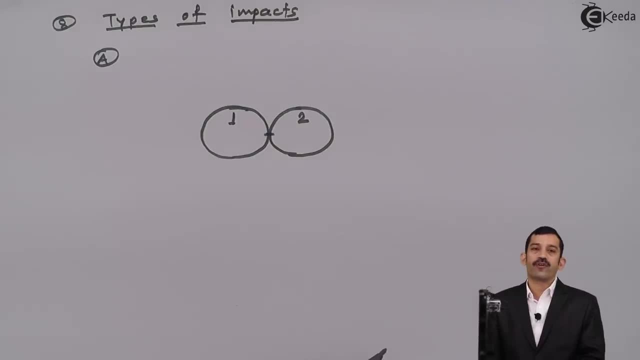 For any circular body. if we will draw normal to the circle at any point on its circumference, then normal to the contact surface here or normal to the circle at any point, always passes through its center. Say this is center of body one, center of body two. If I will draw 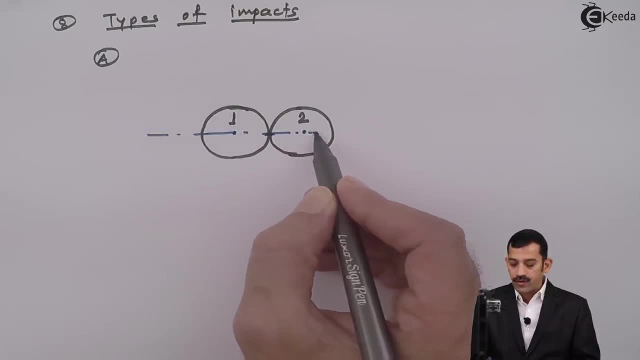 a line which is normal to the contact surfaces during impact. such line is called as what Line of impact? This line is line of impact. That means how we will define this term- New term you can say line of impact- and this one you have to identify while solving problem. 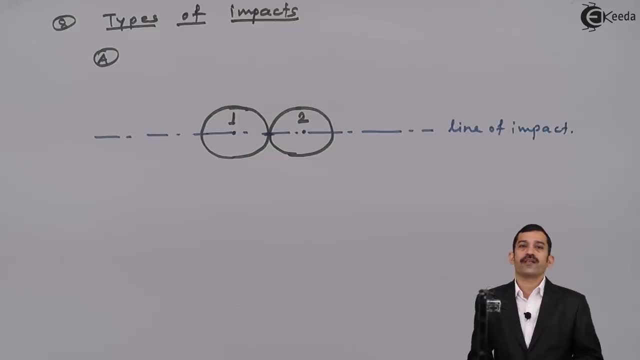 Line of impact is a line which is normal to the contact surfaces during impact. Now, as line of impact is a line which is normal to the contact surfaces, Now, I represented bodies like this. Therefore, horizontal line of impact is possible. That line of impact. 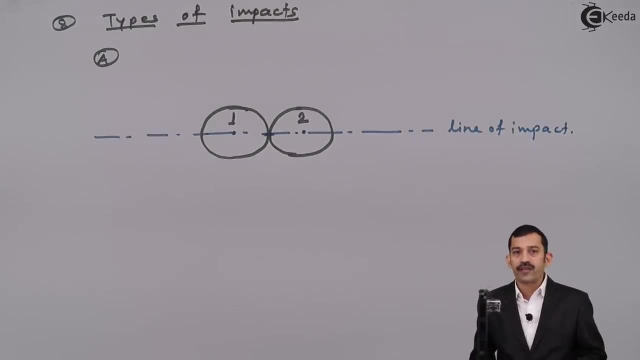 may be vertical possible, Line of impact may be inclined, possible. That depends on what, How, position of bodies is given during impact. Now, as these are the bodies, one and two, If we will represent, If we will assume that body one moves like this Body one moves like. 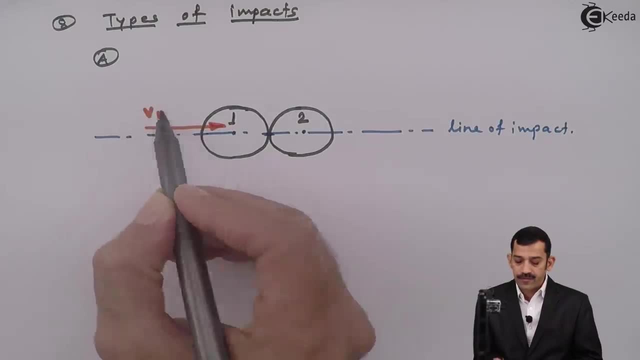 this, So say in rightward direction before impact, say V1. Body two moves in leftward direction. This one is also before impact. That means two bodies are moving towards each other before impact, Just before impact. Now body strikes, Then what happens, Depending. 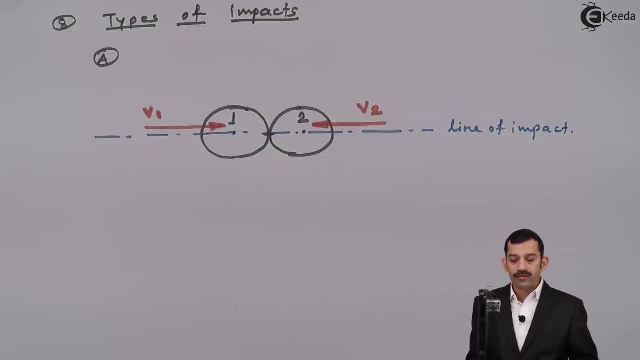 on magnitude of V1 and V2 and depending on masses of the bodies, that body one and two may move in any direction. That depends on masses and initiative. So this is the possibility of velocity. May be possibility is what If mass of body one? 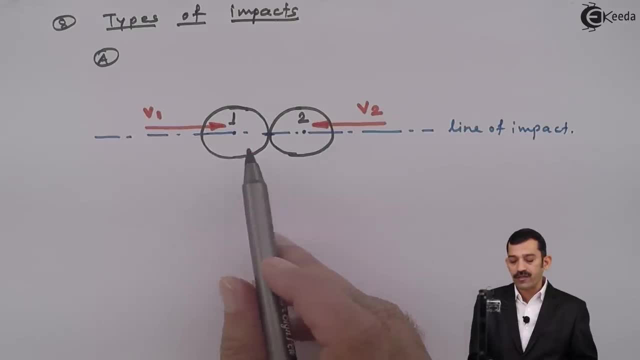 is greater, mass of body two is less. V1 is greater, V2 is less. Both the bodies may move in rightward direction after impact. If mass of body two is greater and V2 is greater, then both the bodies may move in leftward direction. If masses are nearly same, you can say: or there: 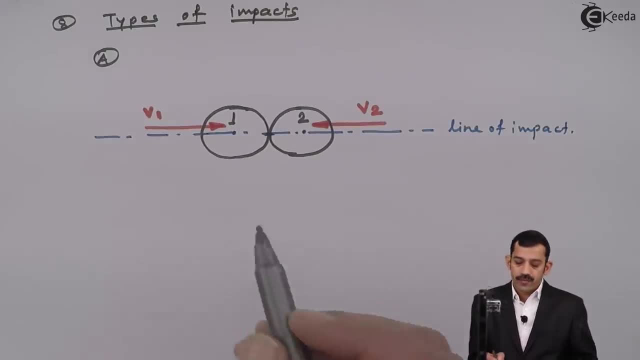 is slight difference. Then, depending on velocity, possibility is what That body one may move in leftward direction after impact, represented by V1 dash. after impact This one becomes what V2 dash. This one is just assumption, Where V1 dash and V2 dash any direction is. 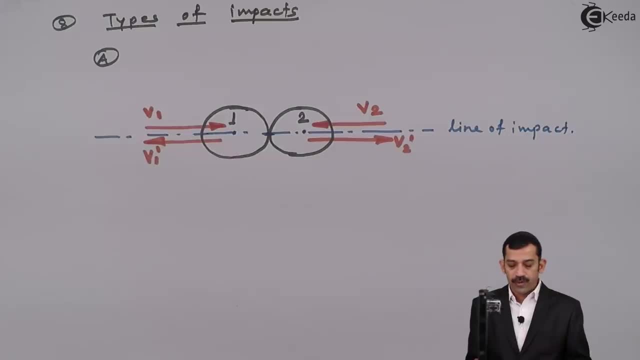 possible, may be rightward, Both may be leftward. What I represented here- first body leftward, second body rightward- Where V1 and V2 represents velocities of bodies one and two just before impact. V1 dash and V2 dash represent velocities of bodies slightly before impact. I have estimated 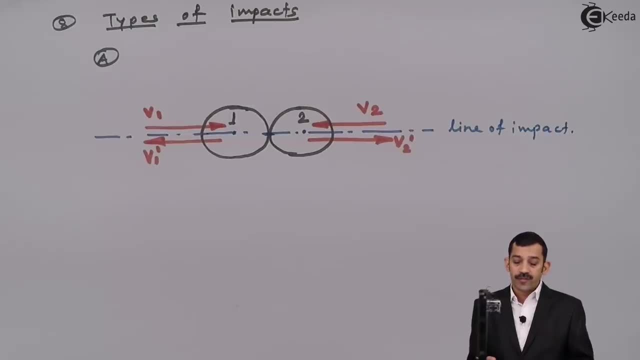 thathee velocity of one body is essence of V2.. So the sub steps of V1 and V2, dash may be different body just after impact. now, when velocities of bodies before and after impact are collinear with line of impact, or you can say parallel to the line of impact, or you can say along the line. 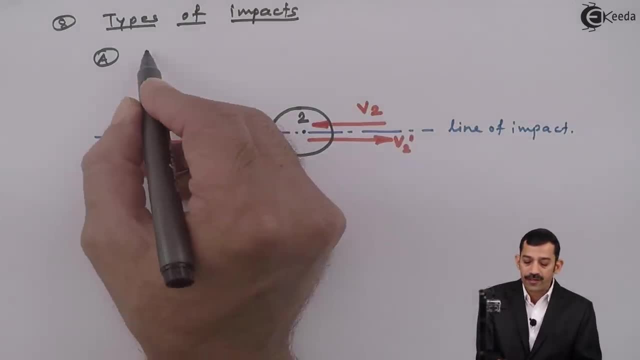 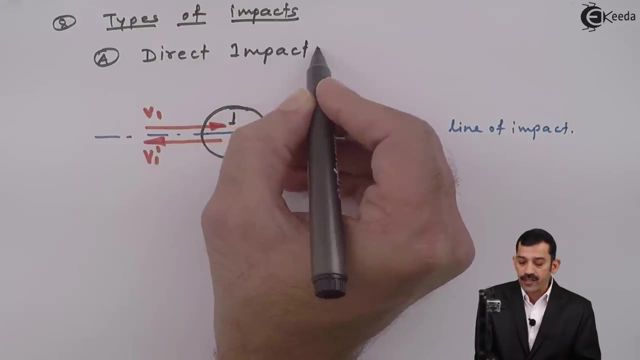 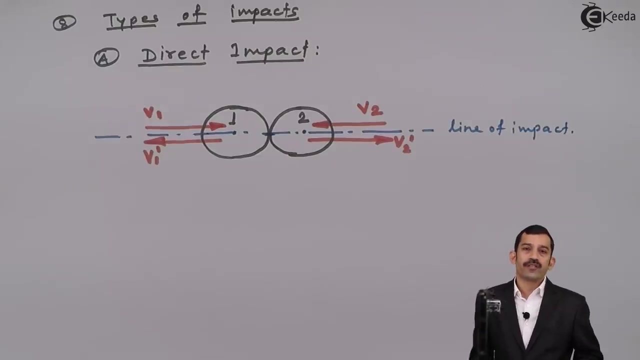 of impact, then such type of impact is called as what direct impact. such type of impact is called as direct impact. that means i will define this type of impact. direct impact means what direct impact is a type of impact in which velocities of bodies just before and after impact are. 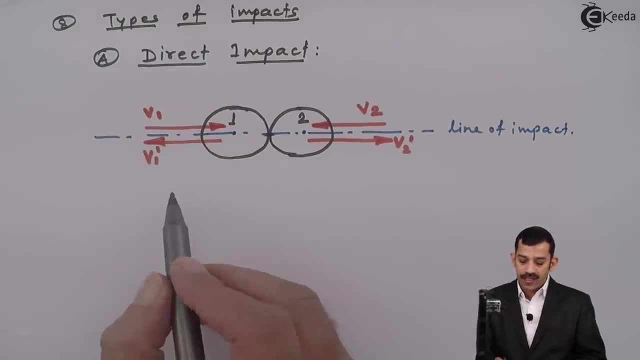 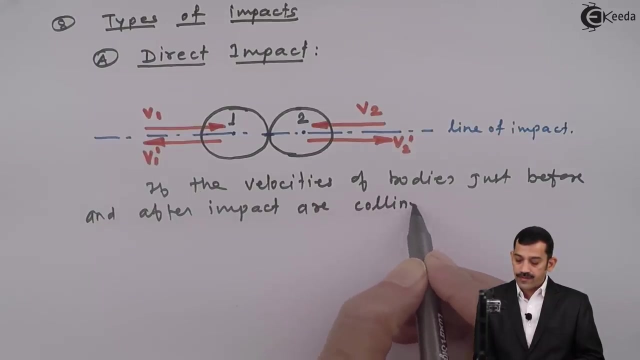 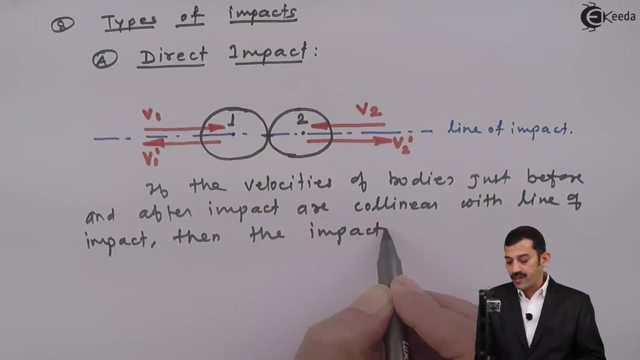 collinear with line of impact, then the impact is called as direct impact. if the velocities, if the velocities of bodies just before and after impact, if the velocities of body just before and after impact are collinear, are collinear with line of impact, are collinear with line of impact, then the impact is called as. then the impact is called. 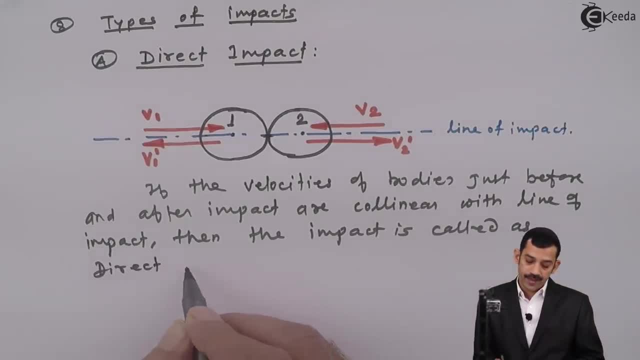 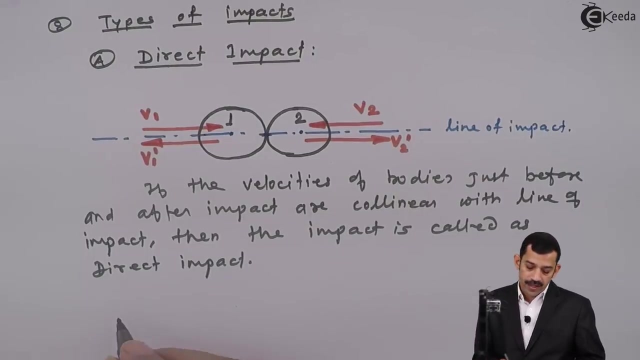 as direct impact. direct impact in the impact is called as direct impact. now for such type of impact- direct impact- our law conservation of momentum and coefficient of restitution is directly applicable. therefore, first, what will get law conservation of momentum? say m1 v1 plus m2, v2 equal to m1 v1 dash plus m2. 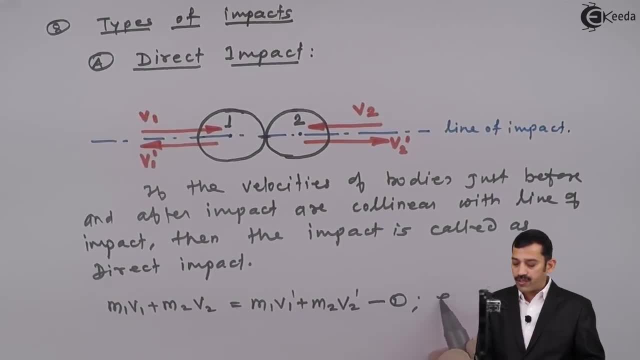 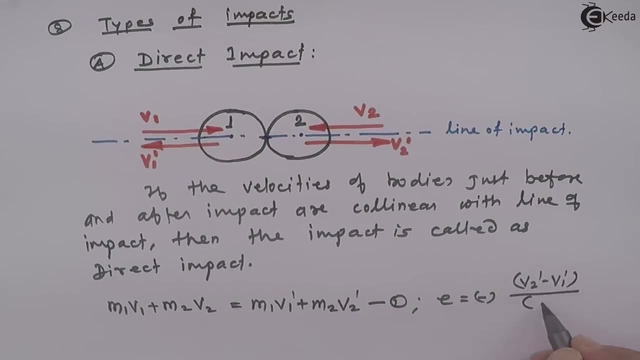 v2 dash. this one is number one. and next, what is we are getting here? is e equal to minus of v2, dash minus v1, dash upon v2 minus v1? both the equations are valid as it is, but condition is what? when? velocities of bodies before and after. 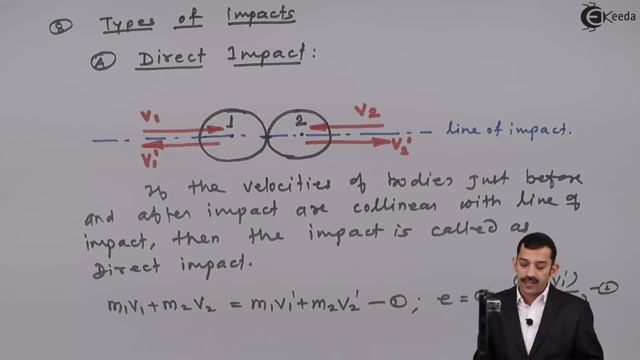 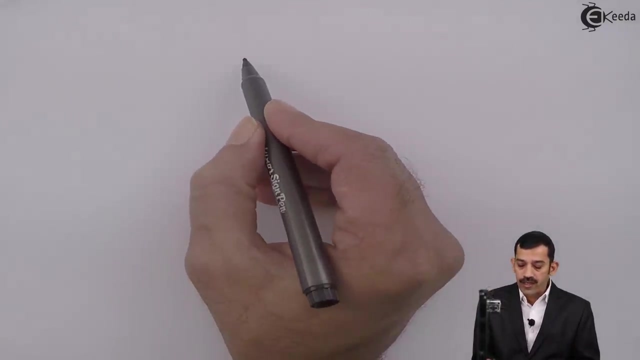 impact are collinear with line of impact, then this impact is called as what direct impact. one more type of impact is possible, depending on direction, of velocity. for example, if i'll take one body like this, this one is, say, body one. now this body one is in contact with 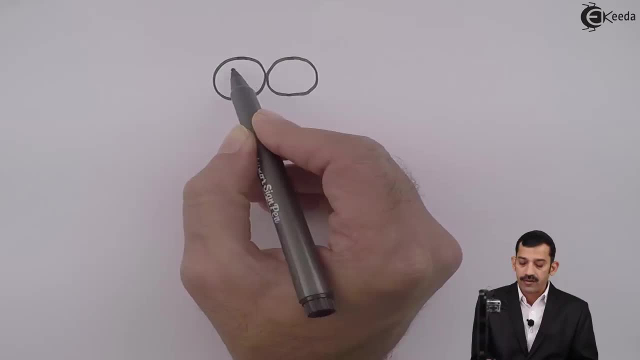 body two again here. that means you know how to represent line of impact. say this is body one, a body two. how will represent line of impact here? line of impact is a line which is normal to the contact surfaces. that means here, if you draw normal that one passes through what centers of 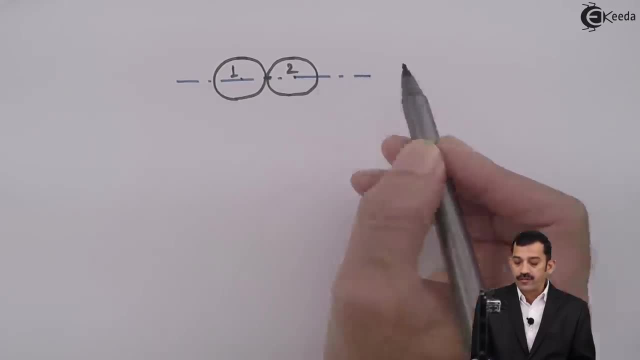 the body. now this one is what this is: a line of impact, right, this line, what we have drawn here is line of impact which is normal to the contact surfaces. so this one is- i'll write as a line of impact: the line which is normal to the contact surfaces is line of impact. now, this body one. 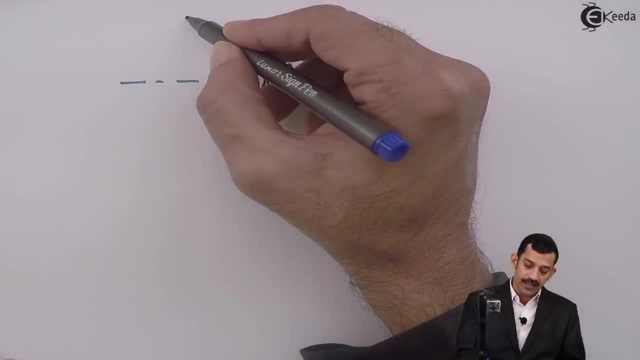 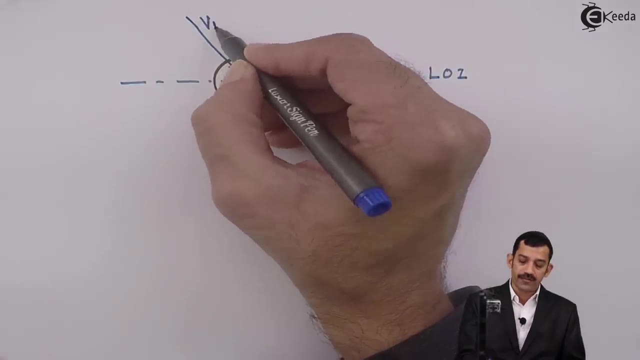 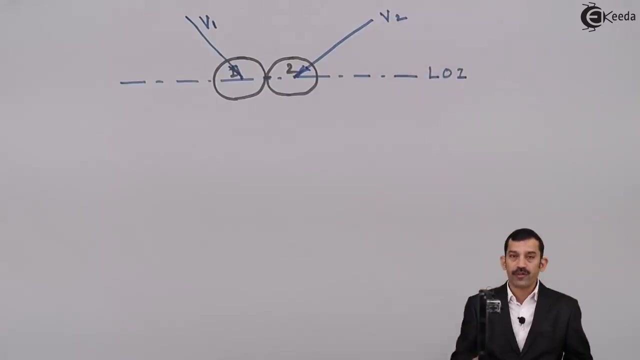 say this: one moves from the direction. this is a direction of motion. body one comes from this side, like this, with velocity v1, and this body two comes from different side. this one is velocity, say, v2. both the velocities are inclined. that means bodies are not moving in a 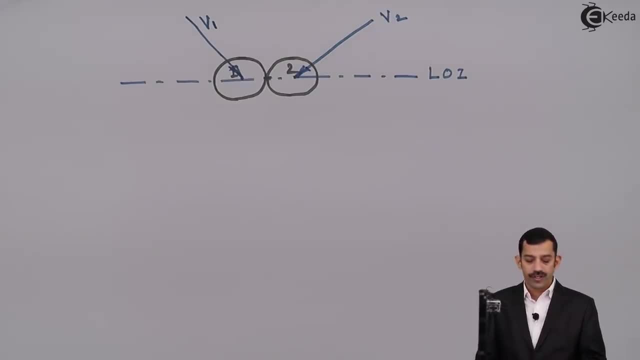 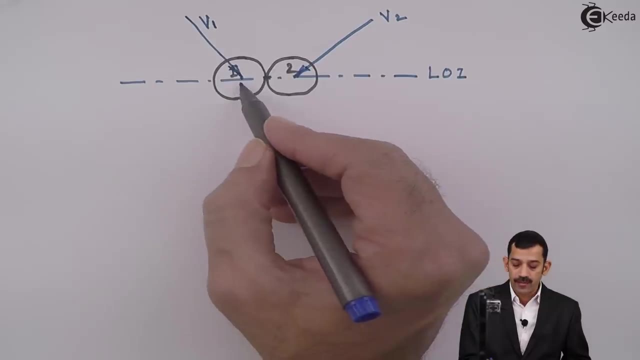 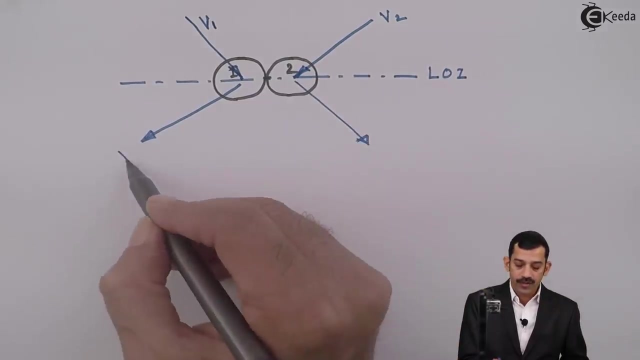 straight, horizontal or in vertical direction. body one moves in inclined direction, body two also comes from some different side. that means, now impact takes place. now what happens? body one rebounds and body two rebounds in different direction. now what you are getting? these velocities after impact, this velocity is also after impact. therefore, v1 dash and v2 dash. now, if we'll see here line of, 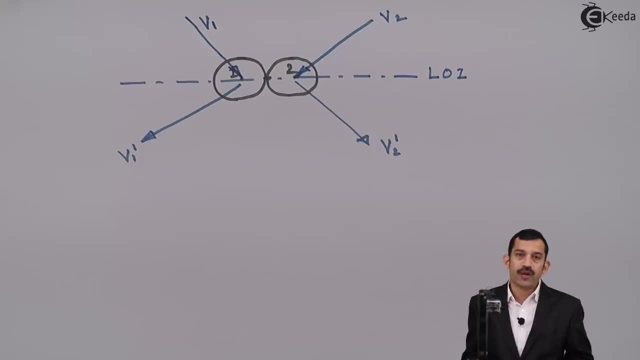 impact and velocities. can we say velocities are non-collinear with line of impact, before and after impact. velocities of bodies are non-collinear with line of impact, then such type of impact is called as what this is. second type is what? indirect impact, indirect impact- let me which type of impact. 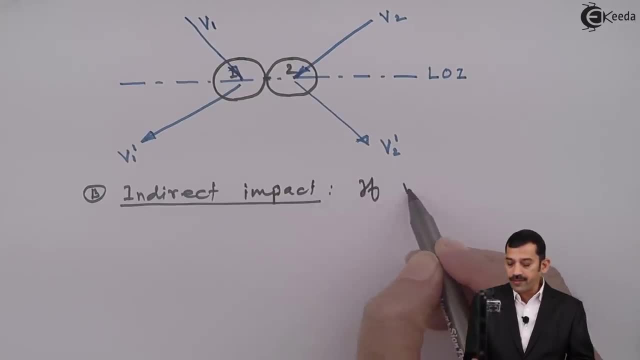 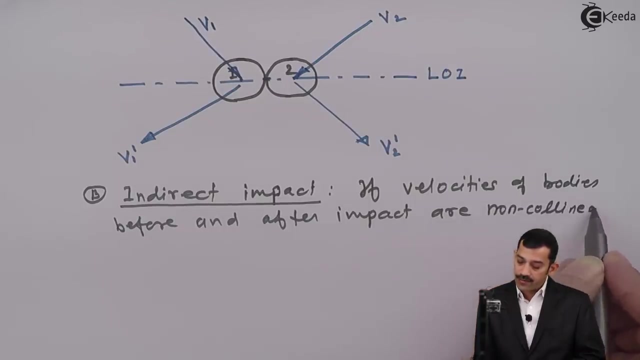 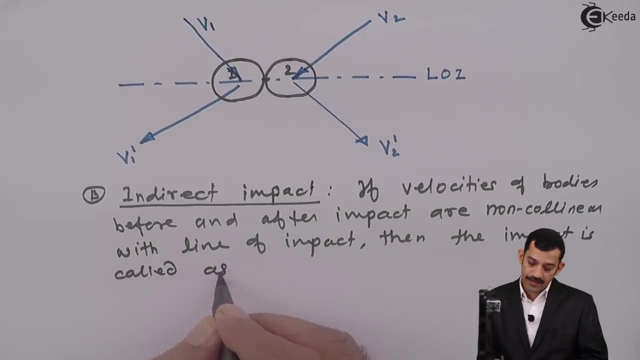 is called as indirect impact. if velocities of bodies before and after impact are non-collinear or non-collinear with line of impact, are non-collinear with line of impact impact or non-collinear with line of impact, then the impact. then the impact is called as indirect impact. 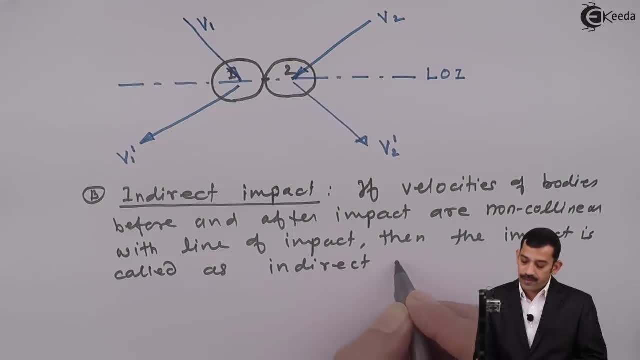 then the impact video flavored movie using springしい 3. the impact is called as indirect impact. Now, in indirect impact and in direct impact, what is the basic difference? In direct impact, velocities are collinear with line of impact. In indirect impact, velocities are non collinear with line of impact. Now, in this one, our equations: 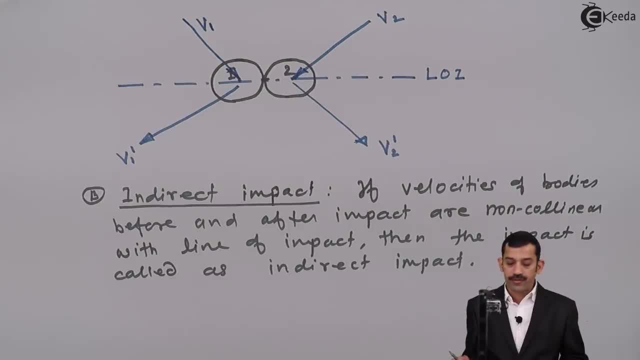 are valid. that means law of conservation of momentum and coefficient of restitution are valid, But when we will apply law of conservation of momentum and coefficient of restitution? this one as it is is not valid. M1- V1 plus M2 V2 equal to M1- V1 dash plus M2- V2 dash. 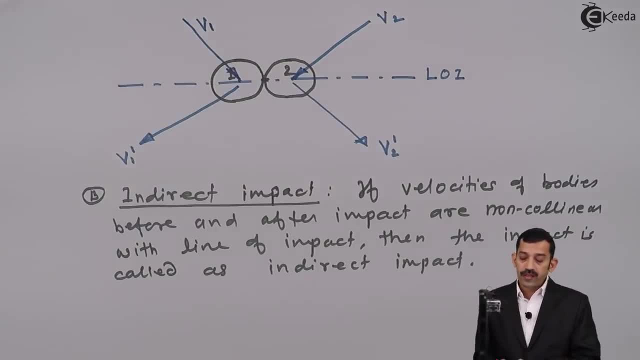 Directly. you cannot apply this equation Here. the components of velocities which are along the line of impact. components of velocities which are along the line of impact, that one varies as per law of conservation of momentum and coefficient of restitution. Only components which are along the line of impact. 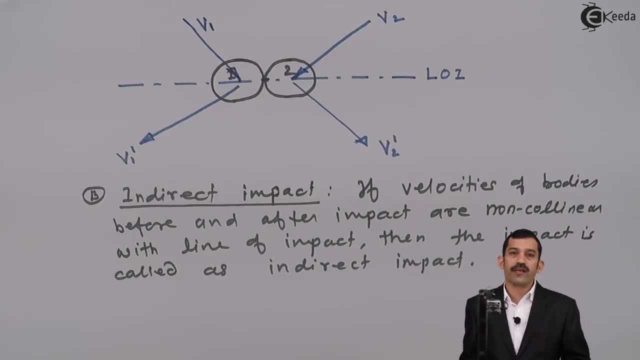 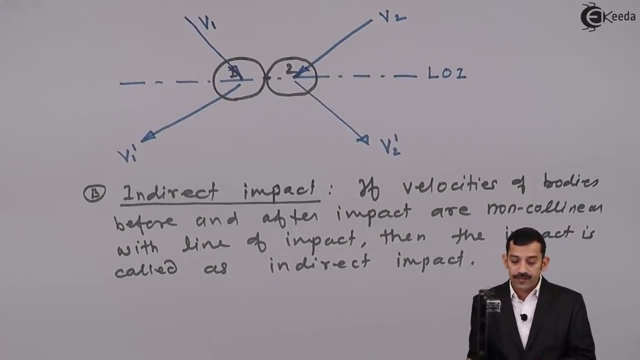 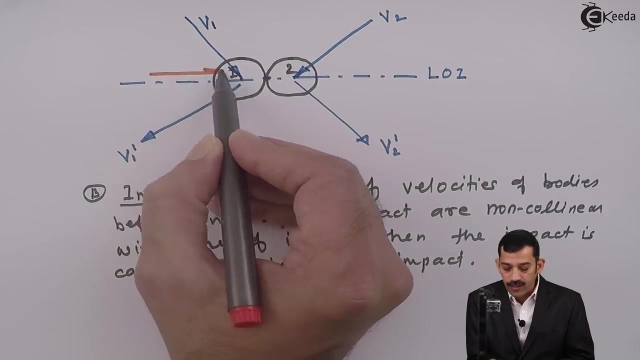 And the components which are perpendicular to the line of impact remains same after impact. That means what it means then. V1 is velocity of body when before impact. That means here, if I will resolve, you will get this component horizontal, this component is what? vertical? If I will resolve, 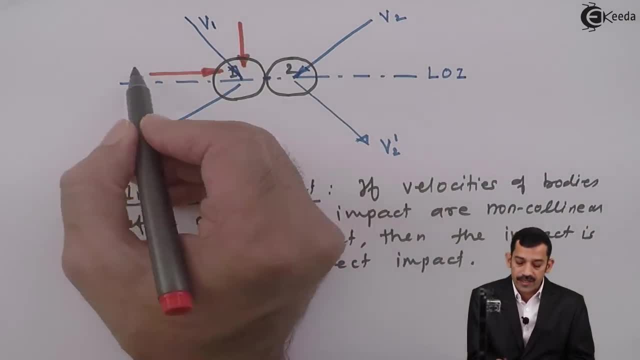 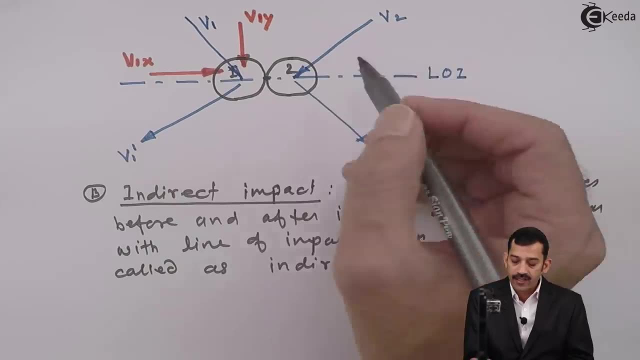 V1 just before impact. That means along the line of impact, say horizontal direction. I will write this one as what V1- X and this one is what V1.. Similarly V2, if I will resolve along the line of impact and perpendicular to line of impact. along the line of impact, what you will get is V2, X and vertical component is what V2 I. 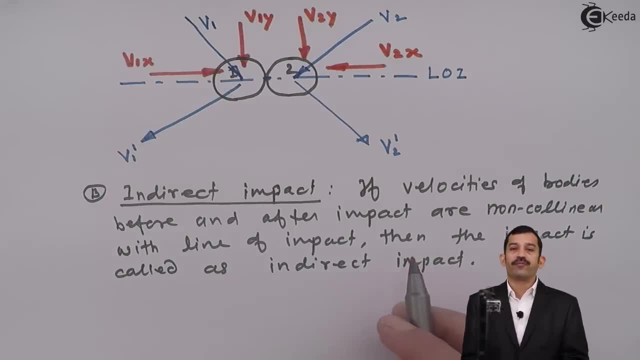 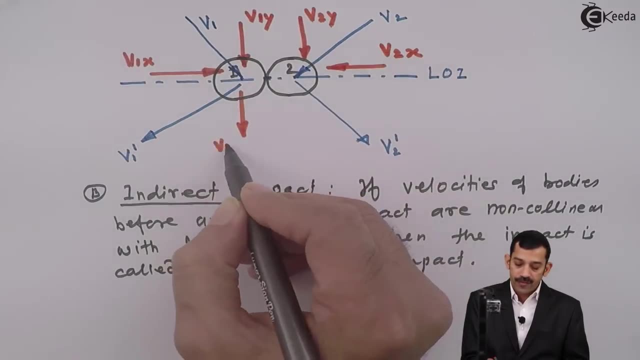 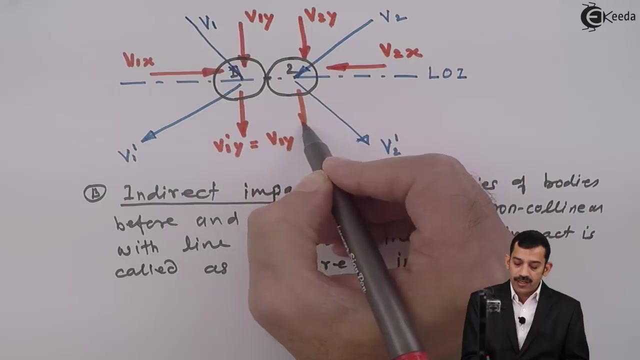 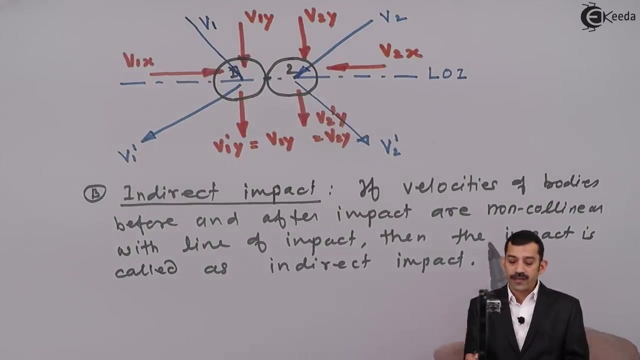 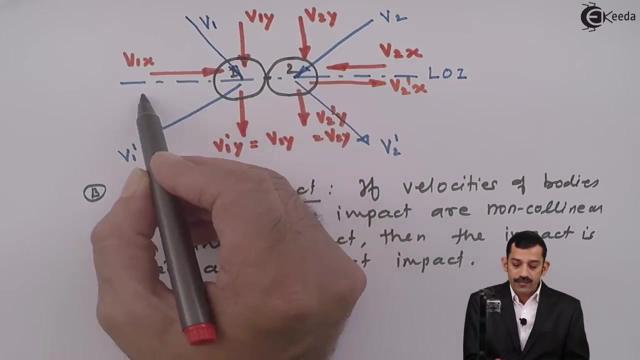 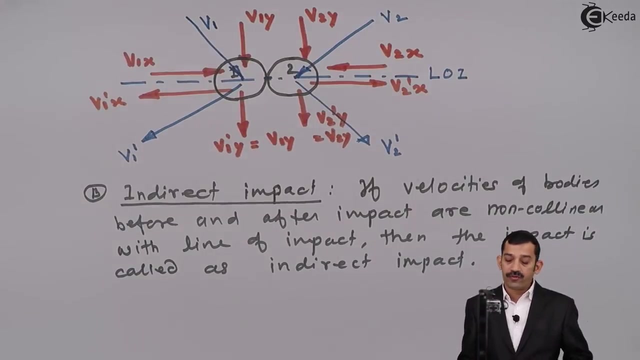 Now, the components which are perpendicular to the line of impact remains same after impact. That means V1 dash. if I will resolve what component you will get here? V1 dash Y is same as that of V1 Y. This component doesn't change. Similarly, this component, what you are getting here is nothing but what V2 dash Y. This is equal to what V2 Y. Component of velocities which are perpendicular to line of impact remains same after impact And other component. that means V2 dash. if I will resolve, will get what V2 dash X, V1 dash. if I will resolve in horizontal direction, what will get here? V1 dash X, That means the components of velocities which are along the line of impact remains same after impact. That means V2 dash. if I will resolve, will get what V2 dash X, V1 dash. if I will resolve in horizontal direction, what will get here? V1 dash X. That means the components of velocities which are along the line of impact remains same after impact And other component. that means V2 dash. if I will resolve, will get what V2 dash X, V1 dash. if I will resolve in horizontal direction, what will get here? V1 dash X. That means the components of velocities which are along the line of impact remains same after impact And other component. that means V2. 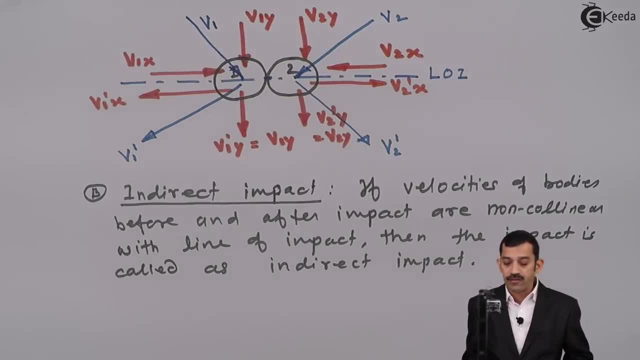 line of impact: V1 X, V2 X, V1 dash X, V2, dash X. These components varies as per law of conservation of momentum and coefficient of restitution equation. That means now for indirect impact. if you want to write these equations- law of conservation of momentum and coefficient of restitution- These equations will get in this component form. If you will write here, just see, Law of conservation of momentum is written as: 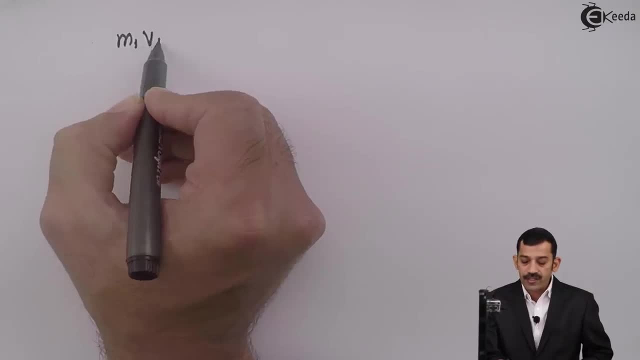 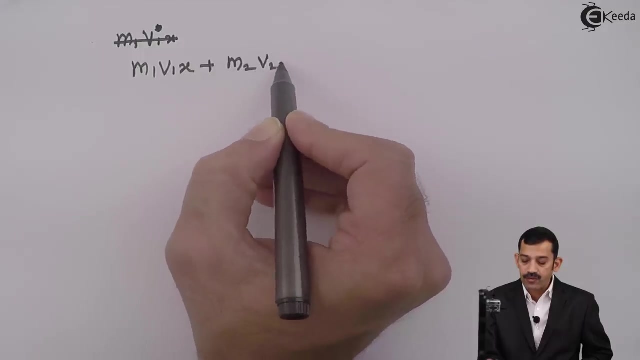 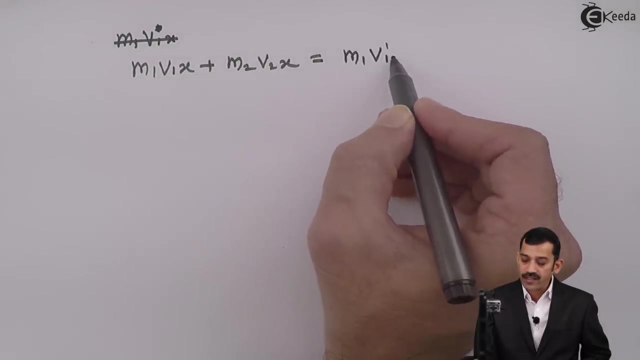 then for body 1 M1, its velocity in horizontal direction, without dash M1 V1 X, again I will write M1 V1 X plus for second body, M2 V2 X. this one is initial momentum. Final momentum is M1 V1 dash X plus M2 V2 dash X. That means you have to. 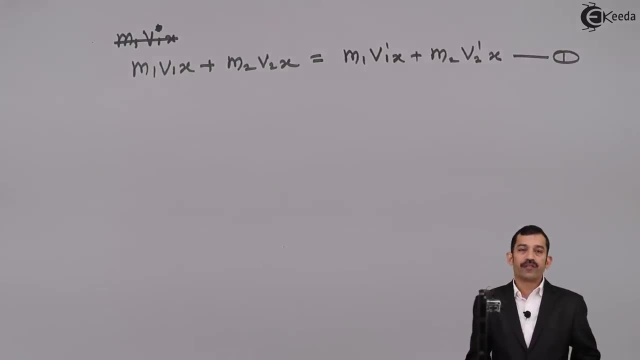 consider which components, Components of velocities, which are along the line of impact Coefficient, of restitution equation. if you will write, it is minus of Now in numerator, initially what we have written V2 dash minus V1 dash, But now it becomes what V2 dash, X minus V1 dash, X upon V2 X minus V1 X. This one is second equation. Now, using this, 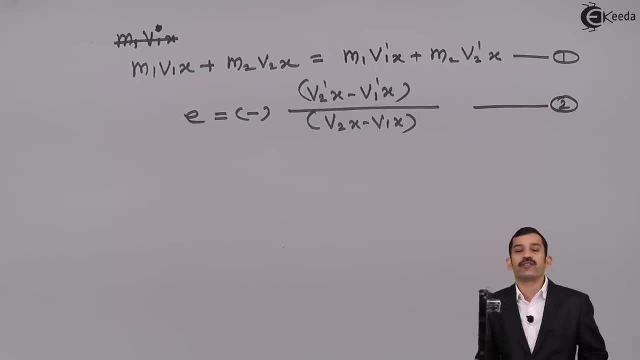 two equations. what will get? components of velocities just after impact in horizontal direction will get. That means solving equation 1 and 2. will find out V1 dash X and V2 dash X, But other components? which components remain same? Components of velocities perpendicular to the line of impact. Components of velocities perpendicular to the line of impact. Components of velocities perpendicular to the line of impact. 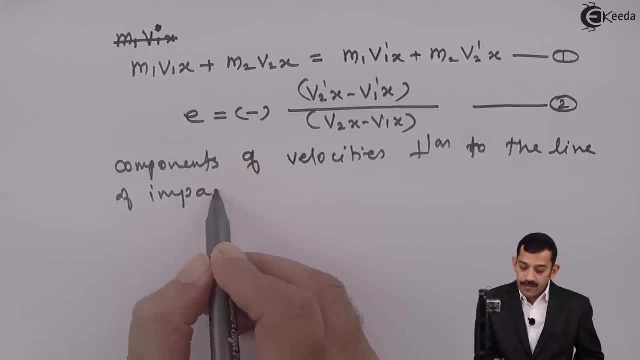 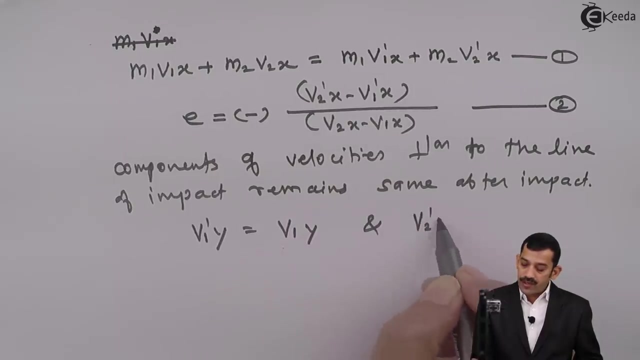 The line of impact remains same after impact. That means, as line of impact is horizontal, vertical component remains same. That means V1 dash Y equal to V1 Y and V2 dash Y equal to V2 Y. That means this one is very important. 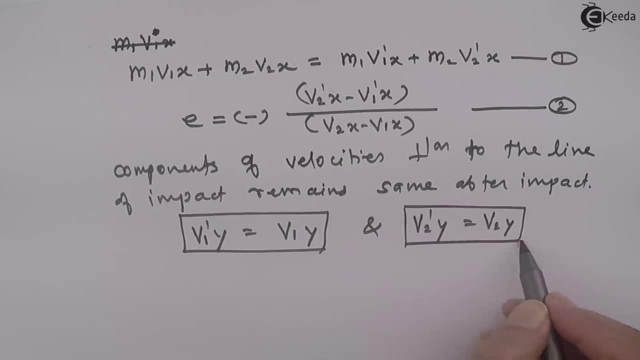 can say: concept one component- that means along the line of impact components- will find out using law of conservation of momentum and coefficient of restitution. the components which are perpendicular to line of impact remains same after impact. therefore, that component remains as it is. once you will get components along the line of impact, applying pythagoras theorem, will find out. 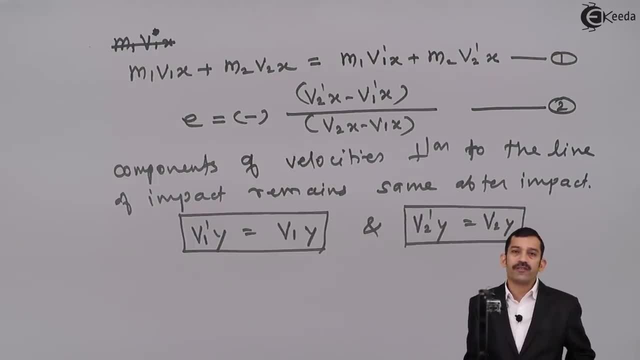 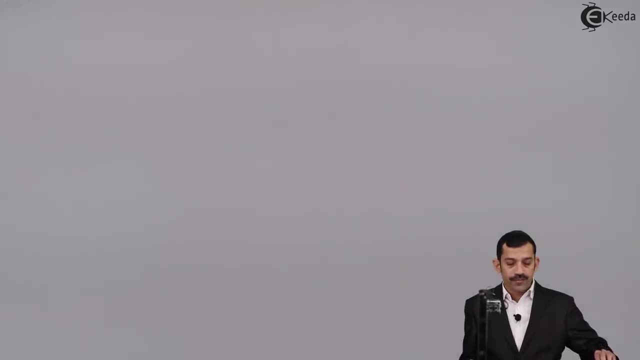 what resultant velocity of these particles just after impact again. next important point is what when two bodies strikes with each other? when two bodies strikes, mass of one body is infinite as compared to other body. that means this one concept is what say point number nine: collision between the two bodies where mass of one part is infinite. can you? 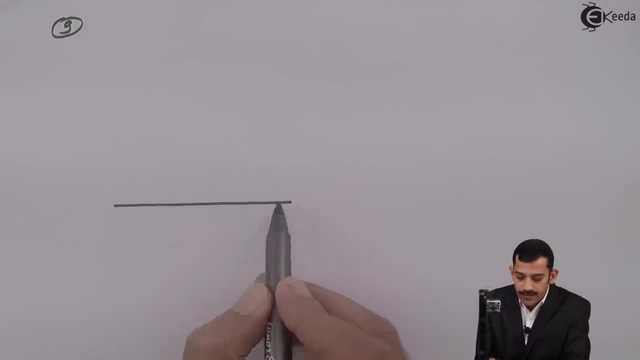 say, say this one is what ground? and here this one is, say ball. now this ball is thrown in downward direction or dropped in downward direction, right, so this ball strikes with the ground. now what is? the mass of ball is negligible as compared to this. one strikes with the ground. 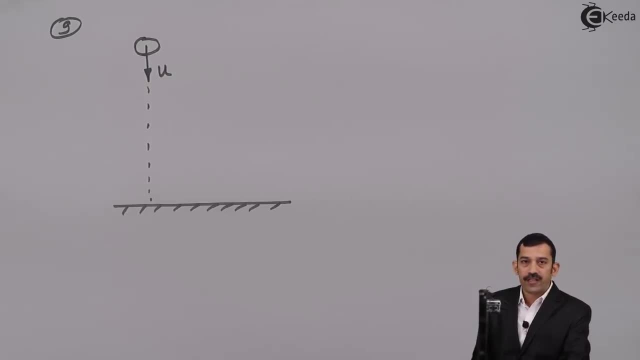 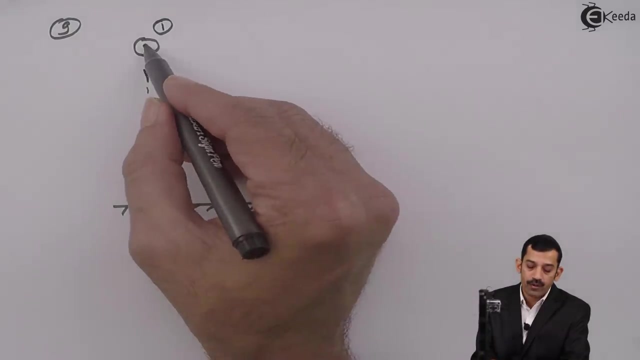 means mass of earth, or mass of earth is infinite as compared to mass of this body. one means ball one. say: this one is body one and what you are getting here, this one is what a ground this one will take as what body two. now, when anybody is thrown in downward direction with 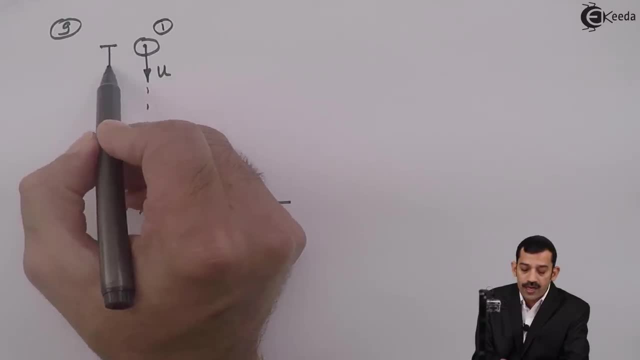 some initial velocity and through some height, you can say h, or may be h 1. if you will assume here what is the velocity with which this body strikes with the ground, that means say what is the velocity? this one and this is body 1, this is the sit, this is what going. 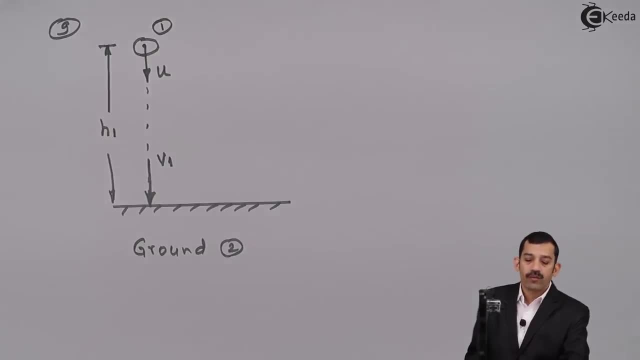 and from here what is? 1? that means how much hijos is this those might take? guys this would take with the ground. that means say what is the velocity. this one and this is bodysy packs. read a lot of speech with this body one. therefore, i will write as what? v1 velocity of body one just before impact. now to find out. 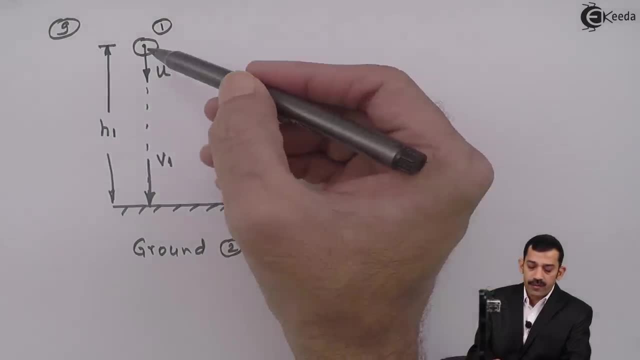 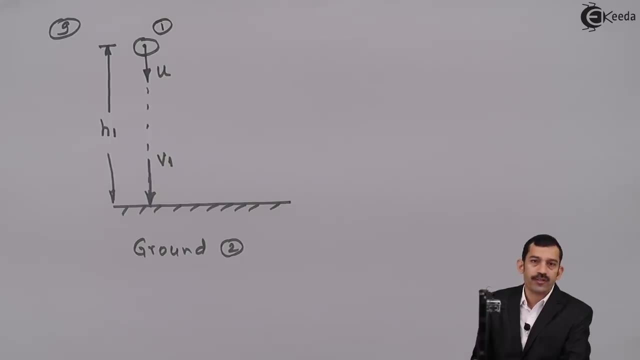 this velocity v1. simple concept: when body is dropped you, if it is zero, then almost you know. v1 is what root of 2gh1. but now it is not dropped, initial velocity is not zero. that means if it is thrown with some initial velocity. so what we will do? we will use law of conservation of energy as 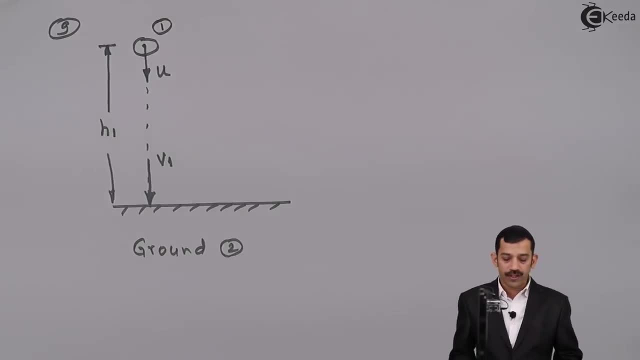 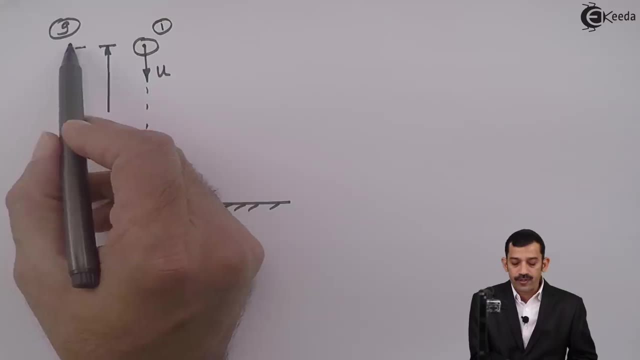 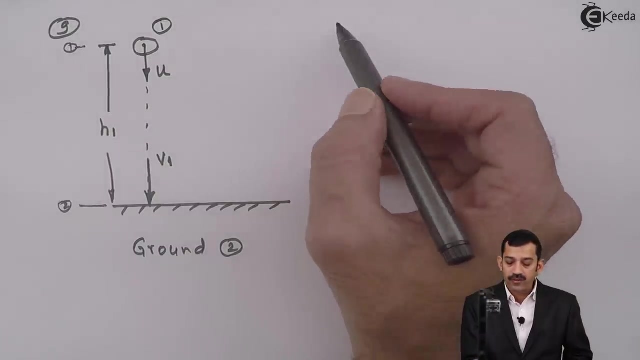 a ball is thrown with some initial velocity, u from height h1, if we will apply law of conservation of energy, say this one i will write as position 1. this one is what say position 2 at position 1. which energies will get to say here? important energies: kinetic energy plus potential energy. 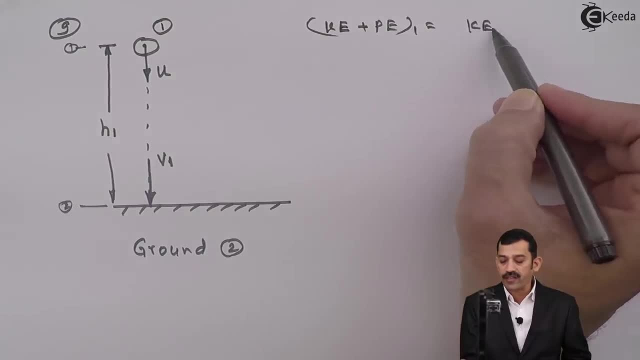 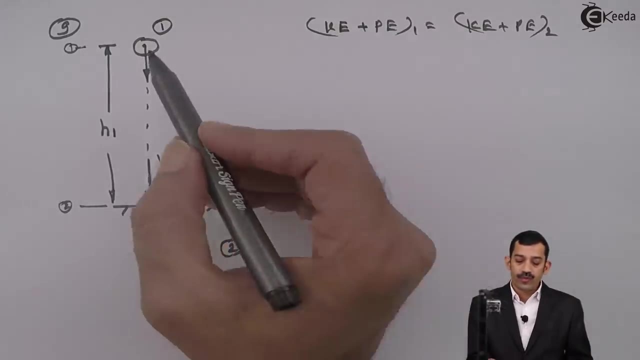 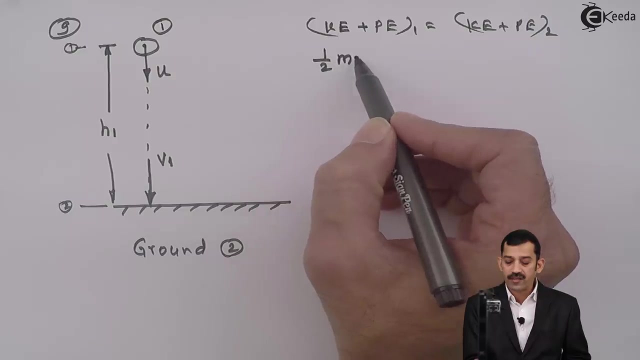 etc. at this position one equal to, again, kinetic energy and potential energy. at position two other energies are not involved. now, at position one, kinetic energy, the? u is given. therefore what will get here half mass into u square? potential energy at position one is due to: you can say: 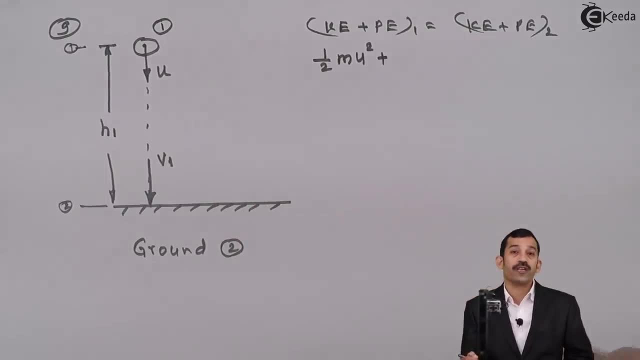 its height. always, potential energy is energy possessed by anybody by virtue of its height. that means this potential energy is what mg h1? now, when this body strikes with velocity v1, that means we'll get some different kinetic energy: half m v1 square. and as it strikes the ground, 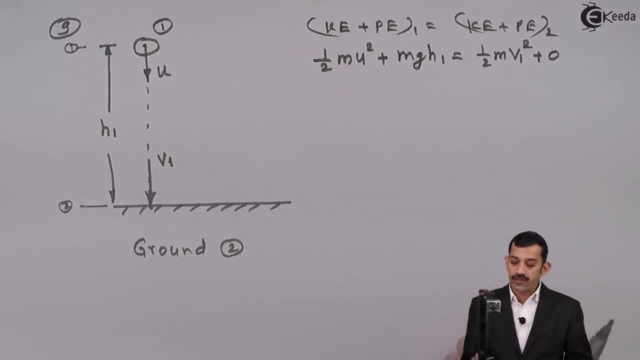 height becomes zero. that means kinetic energy here becomes what? zero. now if we'll cancel this term mass, here mass is same, same body. that means m, m and m equal cancel. now if we'll find out what is now v1 square, 2 will multiply by h2. v1 square. if you will multiply by 2, the water will. 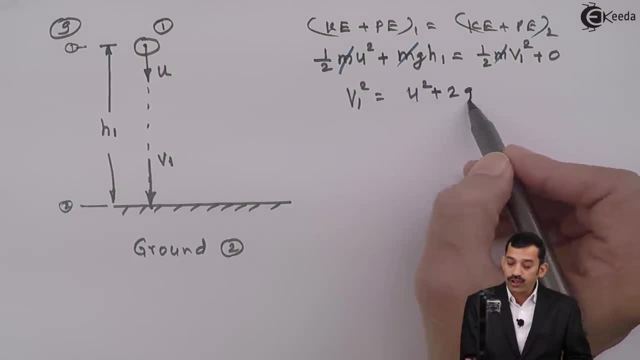 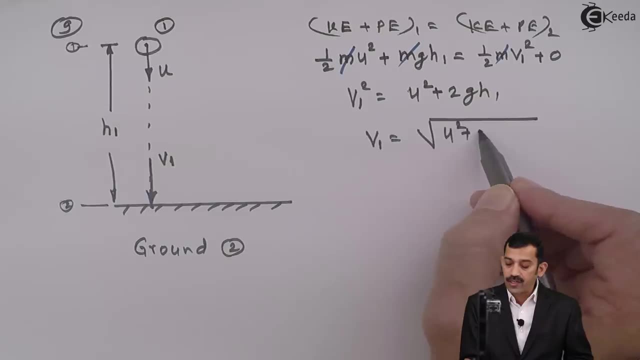 get here u square and again at 2 g h1. that means v1 is square root of u square plus 2 g h1, this one. what will get here? with what velocity body strikes the ground in case if body is not thrown, if velocity of body u is 0 when the body is dropped, if body is dropped, if body is dropped, then 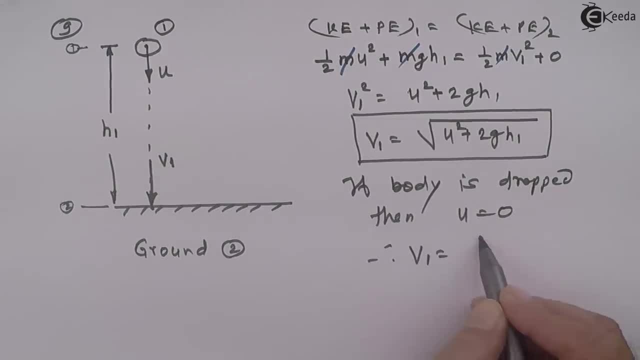 this u becomes 0. therefore this velocity becomes what root of 2 g h1. but if it is thrown, then it becomes what root of u square plus 2 g h1. now body 1 strikes with the ground. what happens? this body will rebound with some velocity and ground remains as it is. that means 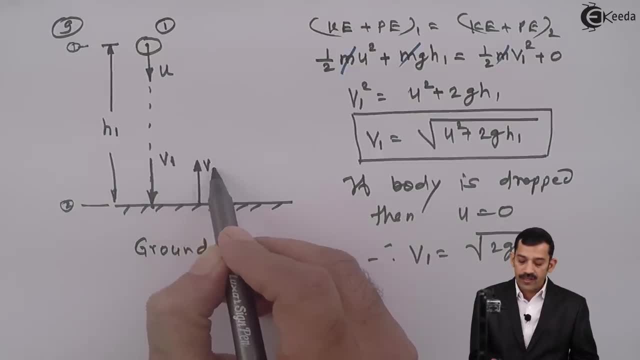 if i'll say this: one is what v? 1 dash, velocity of body, one just before, just after impact. but what about velocities of ground before and after impact here? initially ground is at rest. after impact also, ground remains at rest. that means for ground for second body whose mass is: 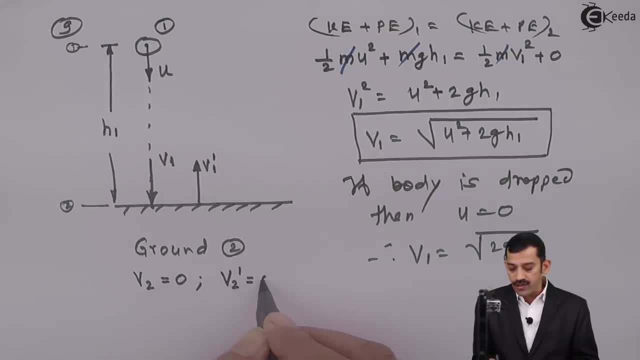 infinite. its v 2 is 0 and v 2 dash is also 0. both the velocities are 0. where you know, v 1 is what root of 2, g, h1. it rebounds with some velocity, as this body rebounds with some velocity, so what? 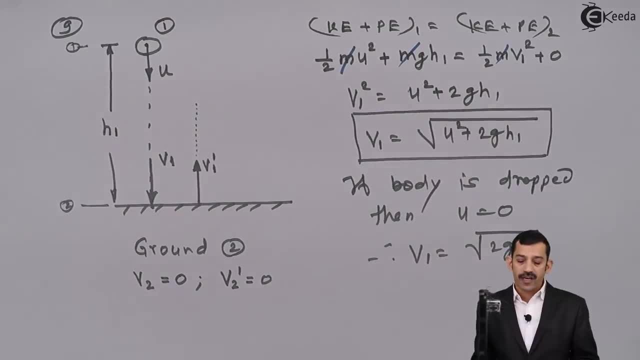 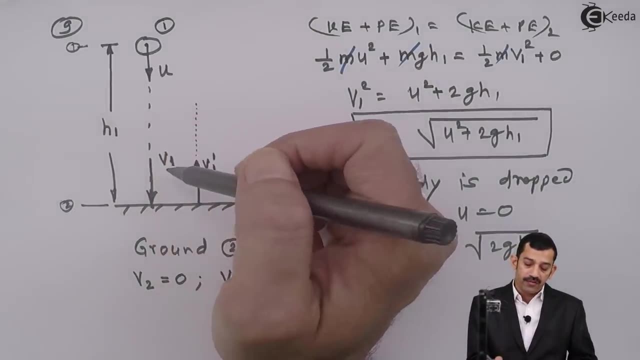 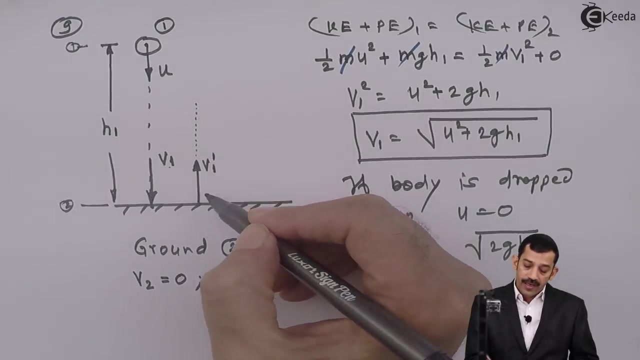 happens: as it moves in upward direction, its velocity gradually decreases and finally velocity becomes 0, as here relation between v 1 and h 1. you know, if u is 0, v 1 is root of 2 g, h1, top 2 g, h1. now, as it moves in upward direction, velocity decreases. and where velocity becomes, 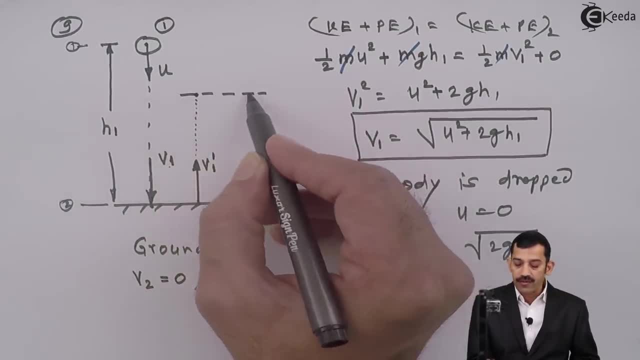 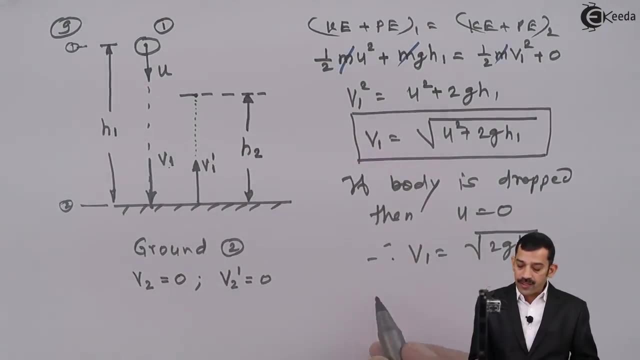 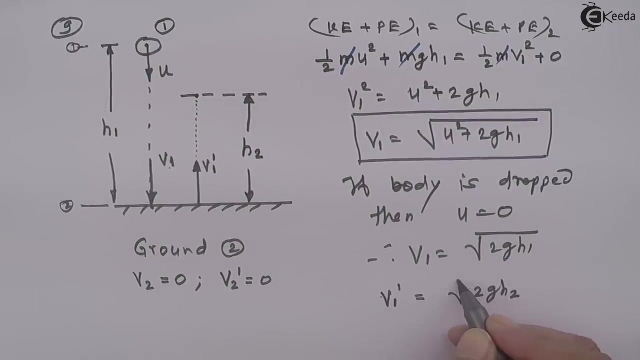 0. can you say here velocity becomes 0. that means what happens here this ball attends. what maximum height? say what h 2 that means what relation between this v 1, dash and h 2 will get to? can you say it is root top uh 2, g, h 2, because here velocity becomes 0. if its velocity doesn't, 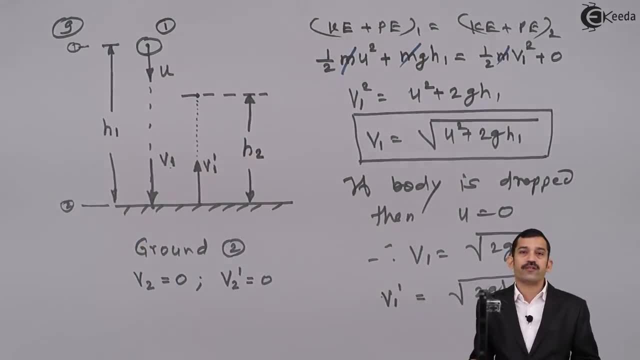 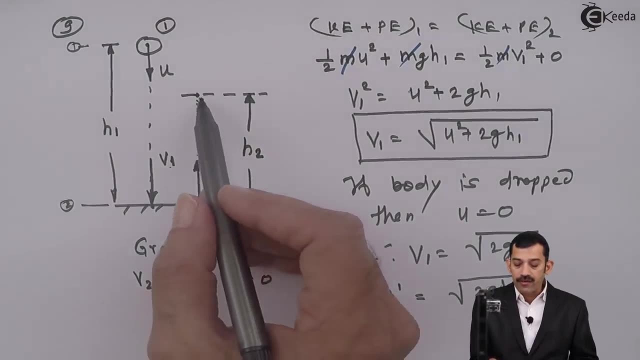 become 0, then root of that velocity square plus 2, g, h 2, is possible. when velocity of ball becomes 0 at some height, that height is what maximum height reached by this ball, just after impact. therefore, relation between v 1 dash and h 2 is what v 1 dash equal to root of 2, j, h 2. now, 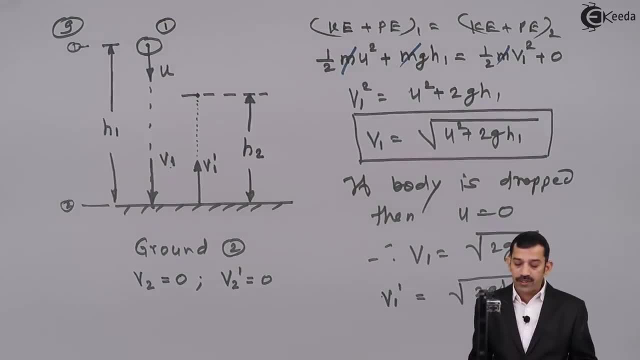 v 1 you know in terms of h 1. v 1 dash, you know in terms of h 2, but we are not considering any sign here. but when we substitute these values in equation, always you have to follow sign convention: upward, positive, downward is what negative that means when we substitute value of v 1? definitely. 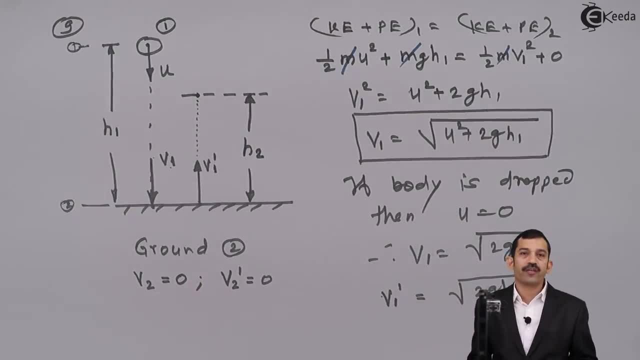 will substitute with minus sign and v 1- dash. if you want to substitute, will write with positive sign. is there any relation between v 1- dash and v 1? that is possible if you will apply coefficient of restitution between these two bodies when these two bodies are strikes. coefficient of restitution. 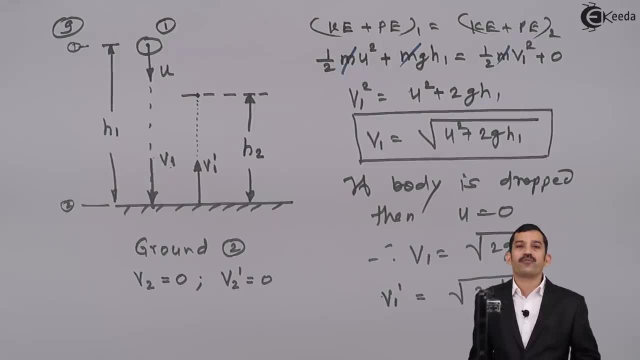 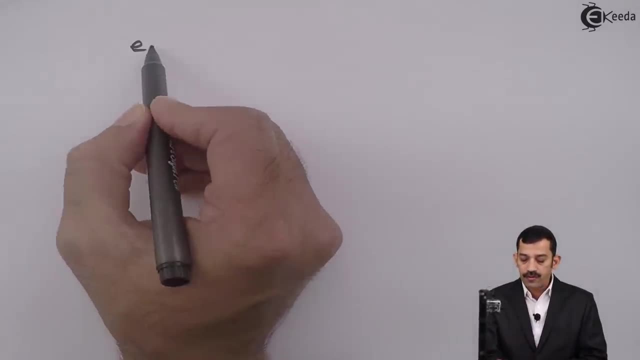 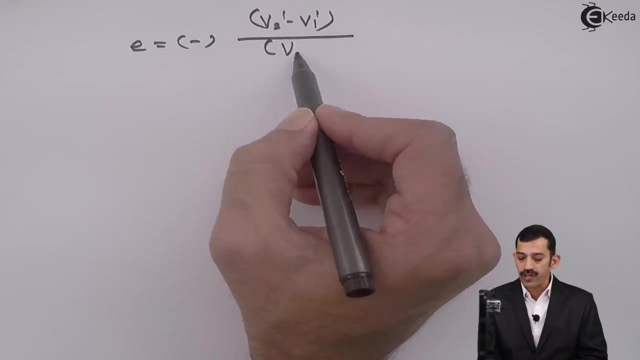 what e equal to minus of v 2, dash minus v 1, dash upon v 2 minus v 1. just see on next page. coefficient of restitution equation is given by v 2 dash minus v 1. dash upon v 2 minus v 1. now here: 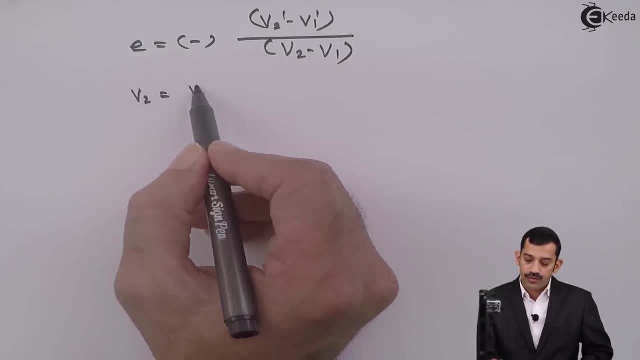 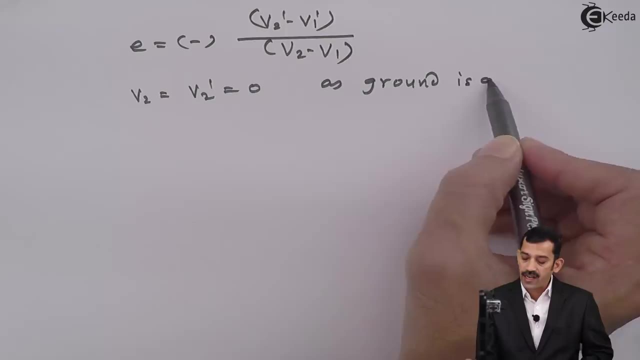 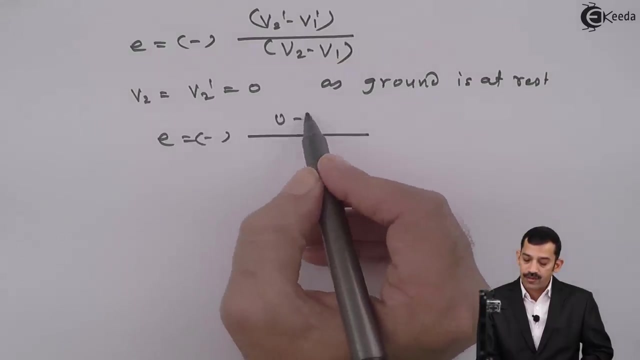 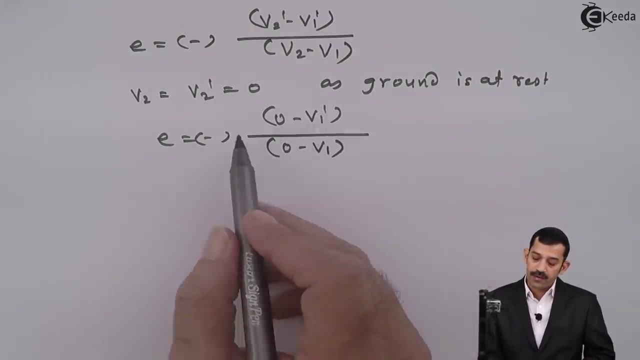 you know, v 2 equal to v 2 dash equal to 0 as ground, as ground is at rest before and after impact. therefore, this e equal to what will get here. e equal to minus of first term: 0 minus v 1. dash upon is 0. what will get here? v 1. that means minus, minus, plus again. 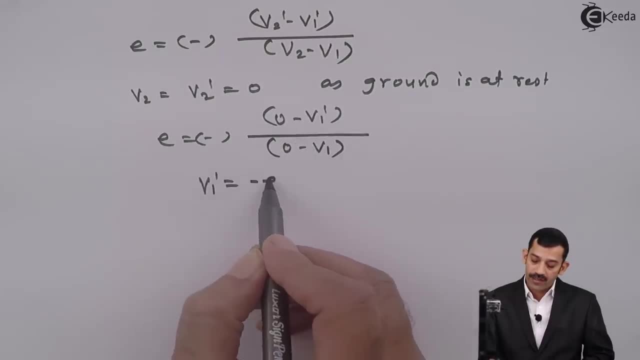 minus mean minus. that means what will get? v 1 dash equal to minus e v 1. v 1 dash equal to minus e v 1. now v 1 dash equal substitute here. v 1 dash is what, in terms of h 2, it is root of? 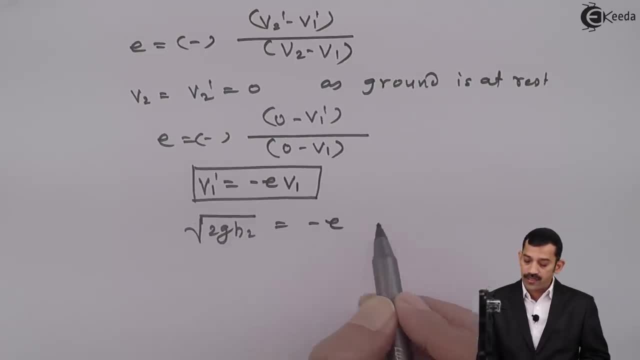 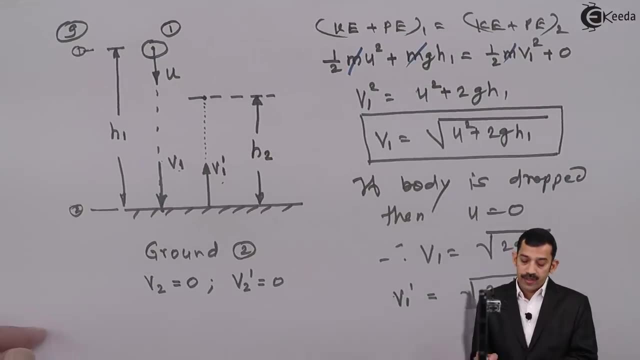 2g h 2 equal to minus e and v 1 is in downward direction. v 1, dash root of 2g h 2, v 1 is in downward direction- will substitute with minus sign and it is assuming it is dropped. what will get here? 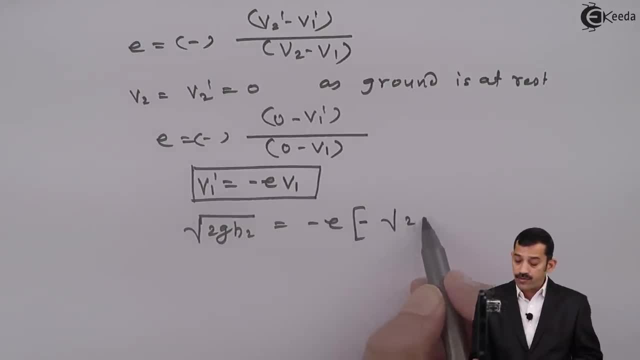 root of 2g- h 1 minus root of 2g- h 1. that means whenever any body is dropped from some height and it rebounds some particular height, say h 2, what relation will get between h 1 and h 2 is equal to.